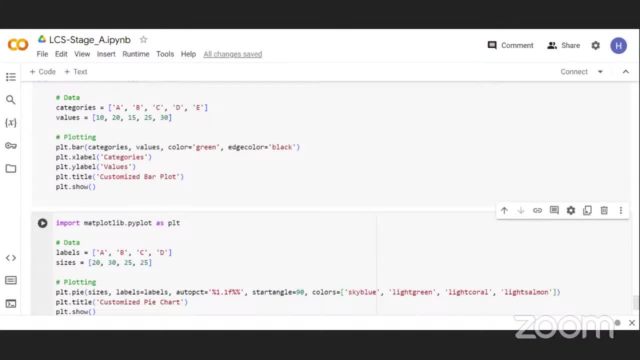 coding session of the current stage. Hi everyone, good evening. My name is Oulabi Adeneo and I welcome you to the last live coding session of the current stage. oh sorry, can you guys hear me now? can you guys hear me now? you can hear you loud and clear. yeah, so we're taking a series of different 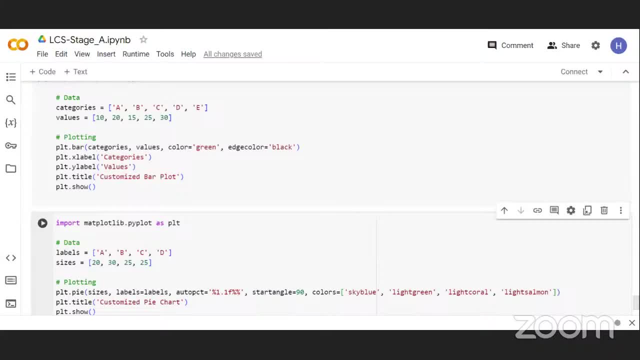 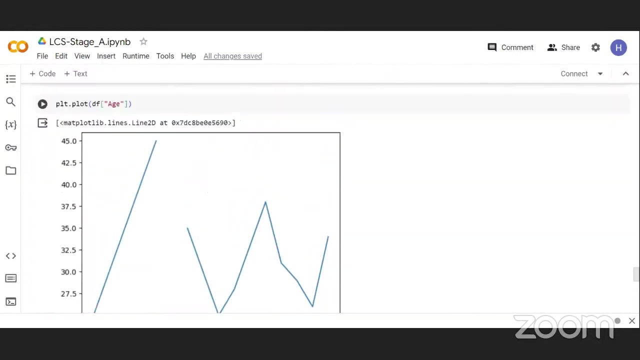 visualizations, taking a series of different visualizations to try and showcase um how we can use pandas in um real world scenarios. so i believe you can see my screen and um, i'll just be picking it up from where we stopped last. so in the last live coding session we just i just showcase the simple manner. 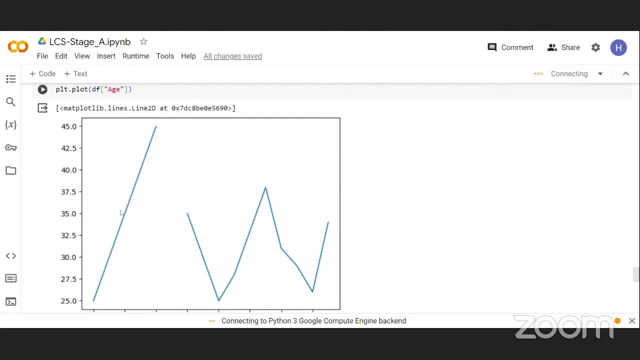 where you can plots, we try to plot a line plot of the different ages that were existing in the data set at that point in time. so today we're showing all of this and then i'm trying to go through each line of code and what each line of code does. 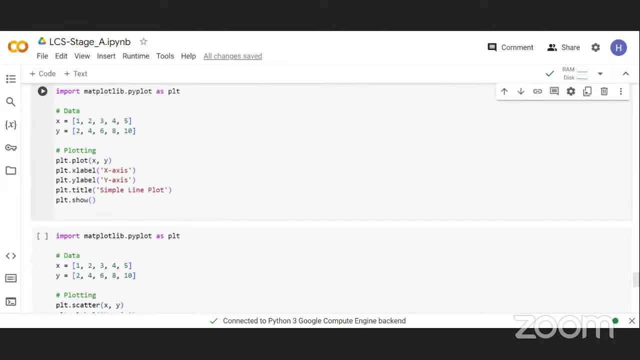 as we are plotting. so the first plot to be showing is the bap, is the line plots, and then, just as we did for the last time, we use plc. so instead of us to keep typing in matplotlibpi plots, we use the um, this variable, to try and shorten the variable name for the imports. so, um, we just is the standard. 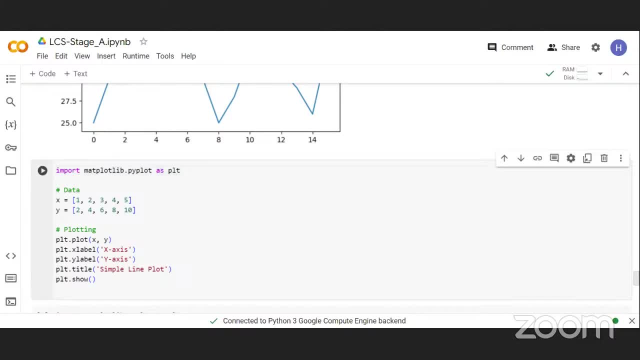 is. you can name it anything you want, but the standard is to always import matplotlibpi plot as plc. so we have two data sets here. the first one is um x variables and then this is y variable, so x and y. so when you use plcplot, the default slot you get using the um pltplot is a line plot. 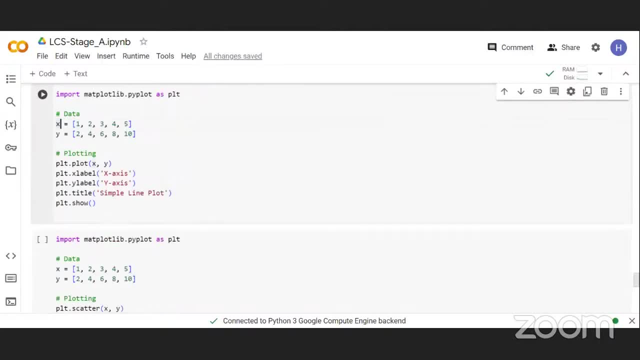 and when you do a line plot, it just basically um tries to showcase what you have on the x-axis and matches it with what you have on the y-axis, and then these two like piece of code. here is what we used to try and label each different axis. so after you make your plots, um matplotlib initial. 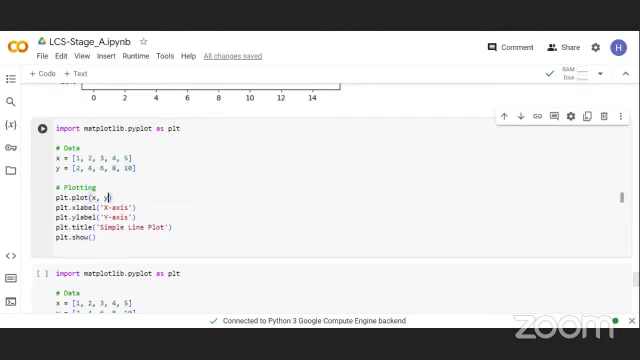 use labels: the plot using the values that are inside whatever it is you are plotting so to give your labels a name. you can use the values that are inside whatever it is you are plotting so to give your labels a name. you have to specify: consider for this plot, all we just have here um 45, then zero. there is no label. 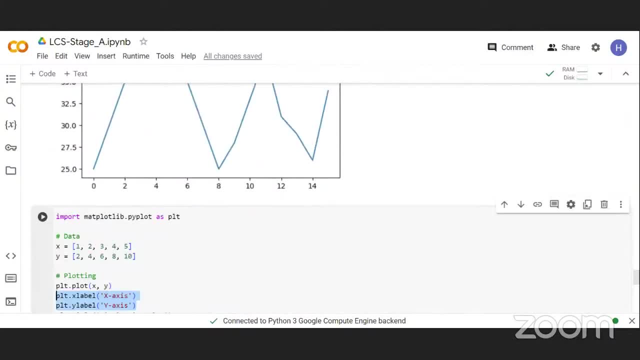 we don't know what is on the y-axis. this is the y-axis, we don't know what is on the x-axis. so to give these values on the x-axis a name and you act as a name, you use these two lines of code here. so 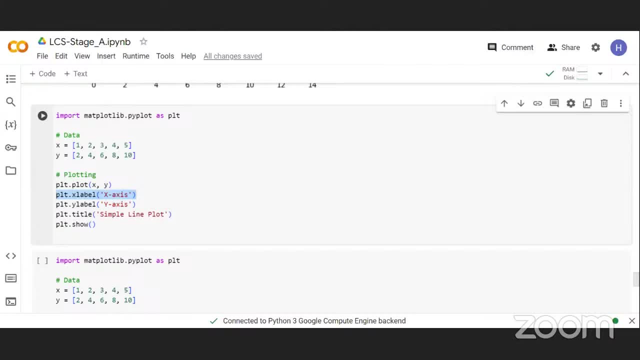 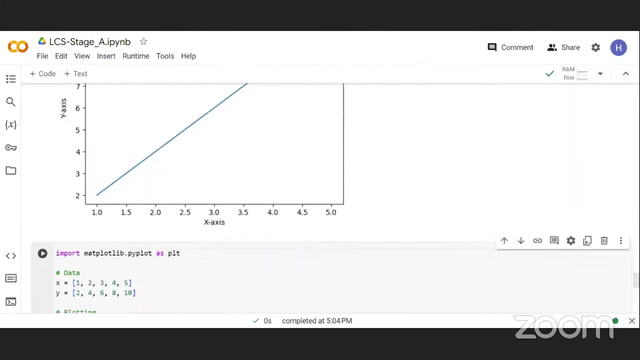 you say you plot on the x that you give the x label. you give the x label an axis, and then you give the y label a name also and then you can also give a title to the plot. so if i run this piece of code now you can see that, um, the y label has been labeled the y-axis. 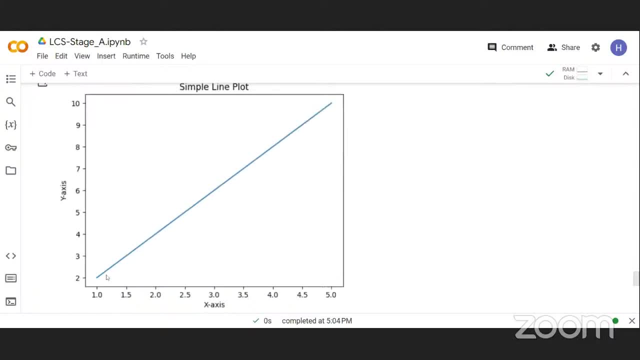 the x label has been related, the exercises, and this is just um a line plot that is matching each x value. so you can see here the value of x is one. when x is equal to one, y is equal to two. so what does that mean? when x is equal to one, y is equal to two. for the next one, um, when x is equal to two, 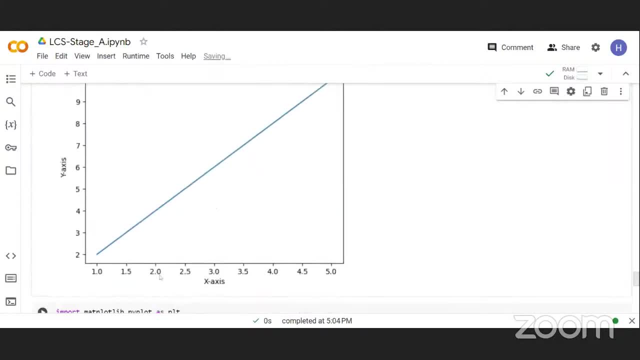 y is equal to four. if you come back to the graph and you try to trace when x is equal to two, you see that way to meet the point, to be at the point where y is equal to four. so this is just a line plot that um matches. 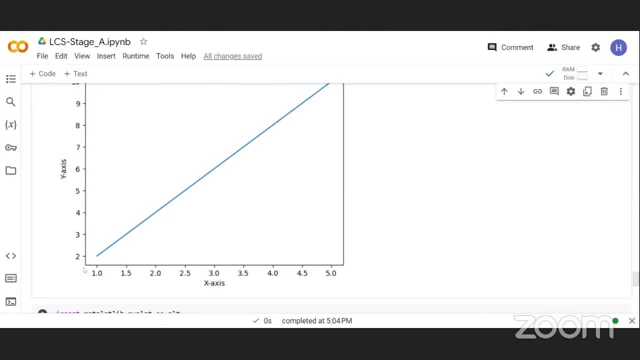 is your x-axis values to your y-axis value and just tries to draw a line that can match each of those values um together in the plot. so that is the basic words, the basic line plots. so a line plot is is a way for you to see the kind of. one of the easiest use of a line plot is to see the. 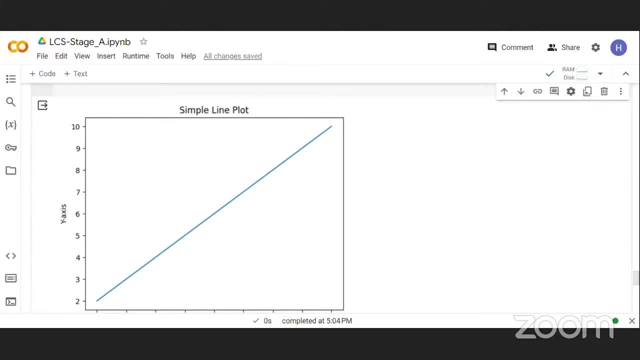 relationship that exists between two. to see relationship that is between two list of values. so for this, now we can see that the relationship is: as x is increasing, y is also increasing. so when x was one, when x was one, y is equal to two. then, at the point where x was two, y became four. 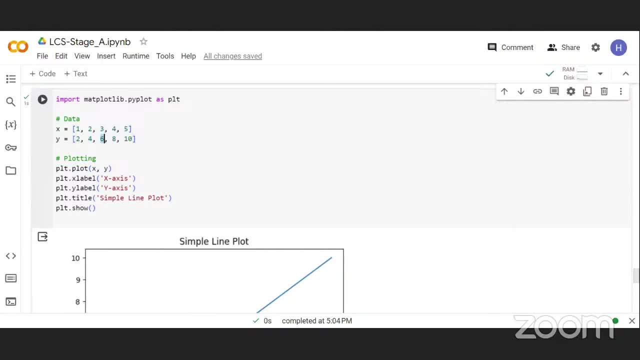 at the point where x was three, y became six. so we can see that there is a direct relationship, that as x is increasing, y is also increasing. so and that is what this line plot is trying to show us. if we try to do the other way around and let us change this and put y 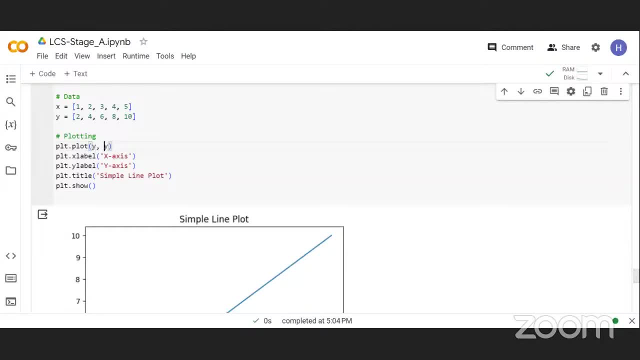 over on the x-axis and put the values of x on this axis. if we regenerate this plot, you'll see that the line is going to show: um, okay, it's showing it down. it's still showing an upward trend, sort of. but what i was trying to achieve is a downward trade where we see that. 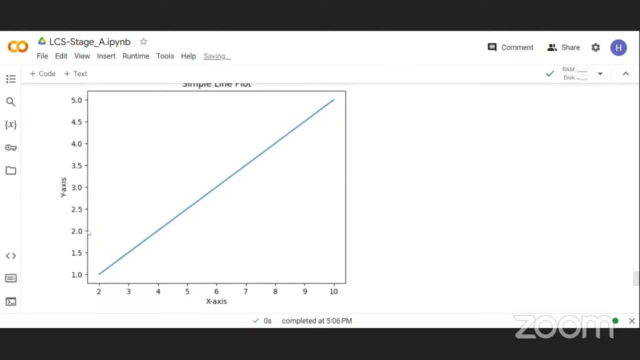 as the values of x, as the values of x um is reducing. okay, is there a way i can do it? okay, let me just try and do something like this. so why dots? let me try and sort this. why dot sorts? okay, oh no, let me just use s-o-r-c-e-g. 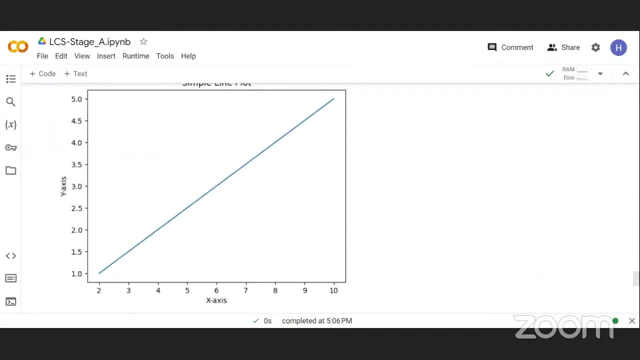 why, i don't know. you just give me so it is t. it is still giving me the same thing. so i want to try and show a line where, um, this line is not going to be drawn this way. it's going to show a variation that comes downwards, so as x-axis. 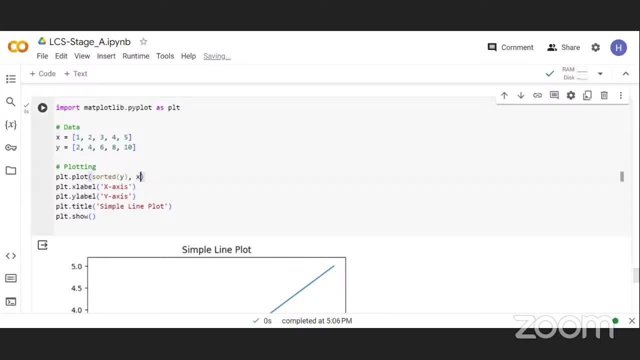 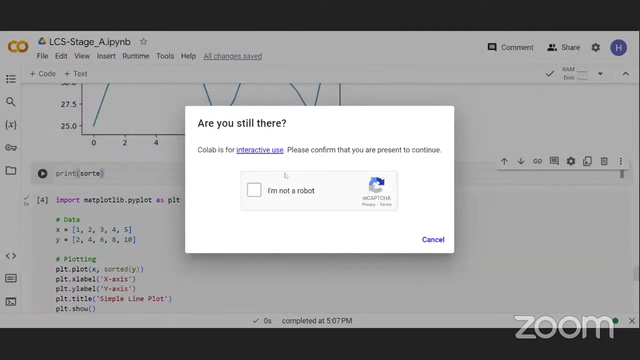 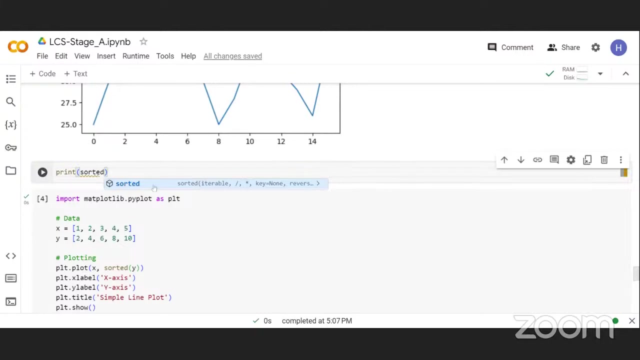 is going to turn. okay, let me see, use the x. let me see when x is equal to one. now, this is not sorry. let me print out this sorted y. so i have to do something where printouts. oh, so i think i can see exactly stirring. then i should be able to say reverse. 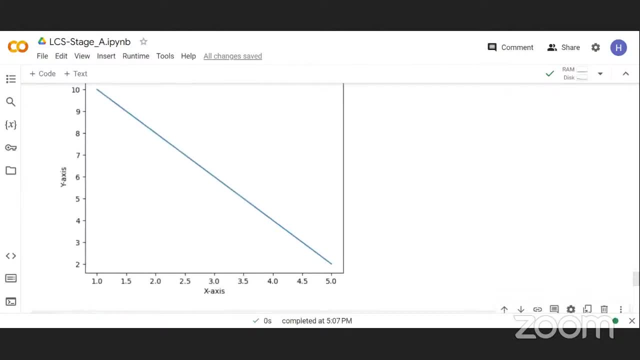 is equals to true. so you can see now that now the line plot has changed from this diaderation, this one is showing another variation that as these values of y are increasing, decreasing, rather the values of x are increasing. so this anniversary spaceship, so when when x is equal to 5, y is equal to 2. when x goes down to 4, then y is equal to 4 when x goes down. 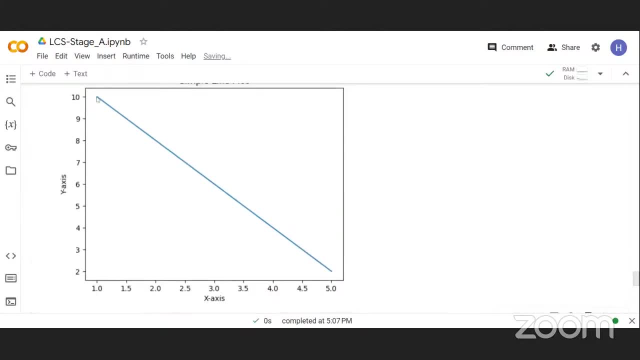 at the point where x is at its lowest of 10, y that is highest of. sorry. when x is at its lowest of 1, y that is highest of 10. so these are ways where you can start to see um the visualization of the relationship that is existing between two variables, using a line plot and then the next. 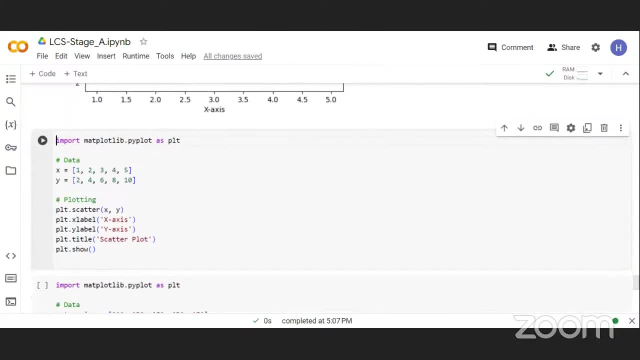 plot that we'll be showcasing is um a scatter plot. so a scatter plot is basically almost the same thing as a line plot. the only difference is that a scatter plot does not try to give you a line, it just gives you different dots that denote um where the x and the y axis meets. so, as you can, 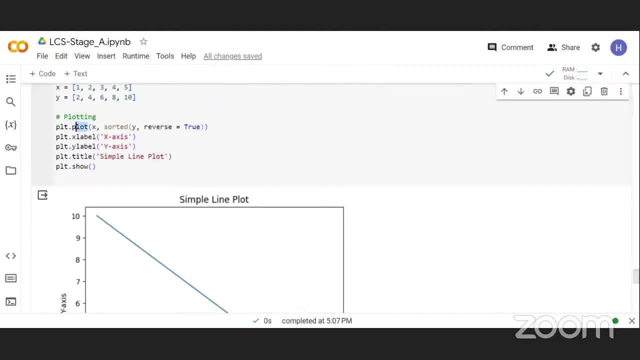 see. the only difference here is in the line plot we use plt dot plots, but here we are using um plt dot scatter. so you do plt, just cut that instead of you having a line plot. the results you have is this: i can see. that is basically the same thing. the only difference now is that we are not drawing a line. 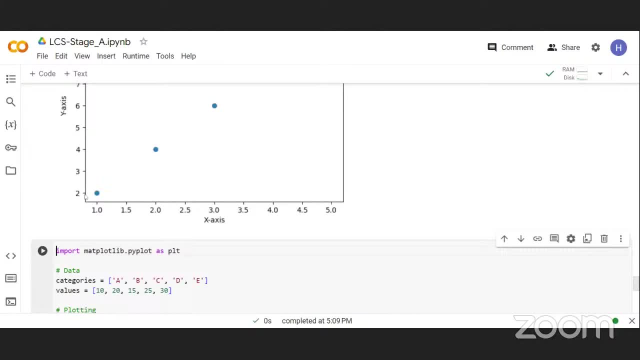 rather, we are showing the points where both of them meet. so, yeah, we are showing that at points one, x is equal to one, y is equal to two. this is the point here. when x is equal to two, y is equal to four. this is this point. i can see that if you try to draw a line, it will get you back to. 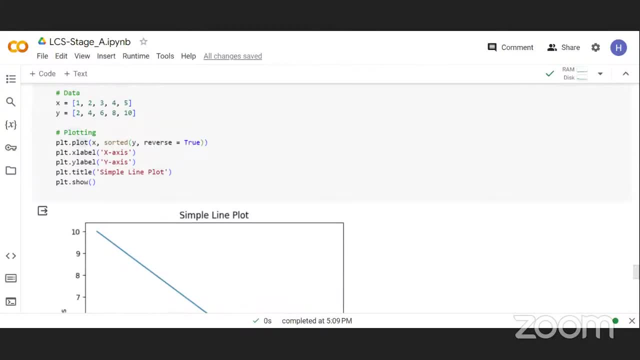 this um particular value here. you also come here here and copy this and i bring it down here and face it here. you see that it's also the same. so it does like nine. at the points where x is equal to one, our y is equals to 10. at the point where x is equal to two, y is equal to 8I. the point x is: 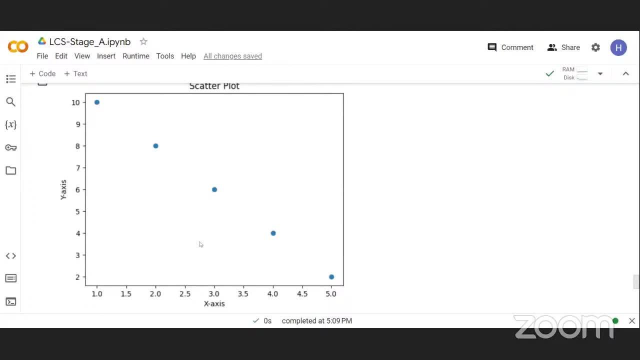 equals to three, um y is equal to 6, so scattered plots is basically almost the same thing. at the 9 plot the only difference is that in your scatter plot it does give you the dot that denotes where the values on the x and the x as and y axis meet. meanwhile the line plot tries to give you is: 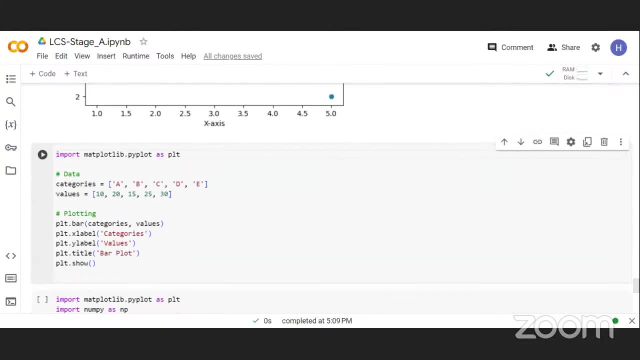 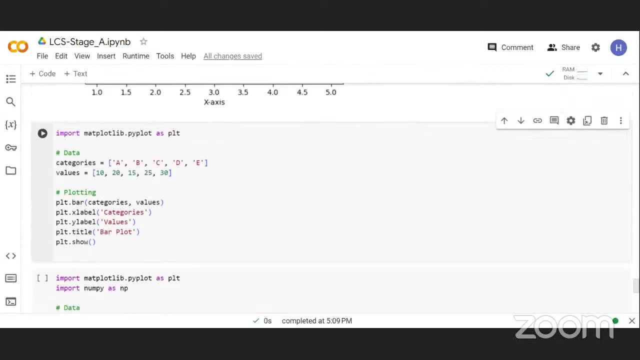 tries to fit a straight line into where these values meet, rather than giving you the actual points. so the next plot we'll be talking about is, um, a bar chart, and we all know what a bar chart is. a bar chart just basically shows, um a list of- uh, different values for different categories, using a 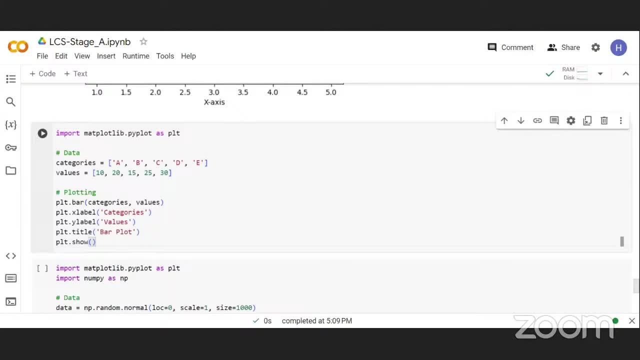 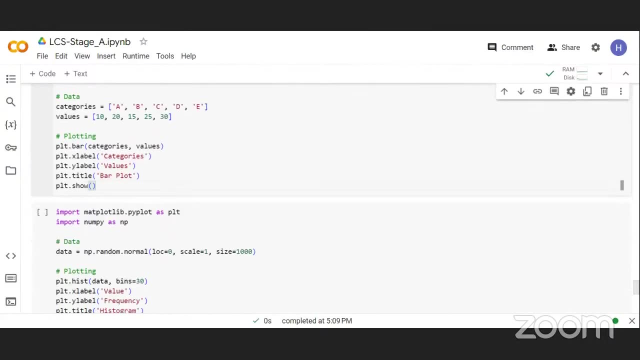 bar. so the higher the bar, the higher the number of values that fall into that particular category. and you can see that the syntax for matplotlib is very simple. we are still using- we've been using- the same thing ever since, the only difference that has been changing, the only thing that has. 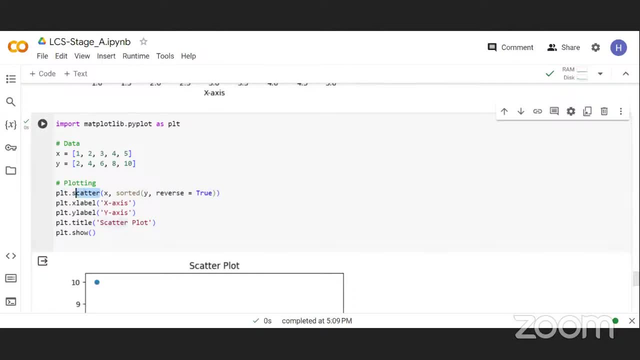 been changing is what the function we are calling for the plt does um the kind of plots. we only wanted the name plot to use plt dot plot. when we want the scatter plot to use plt dot scatter, now that i want a bad plot, we are using what's plt dot bar. 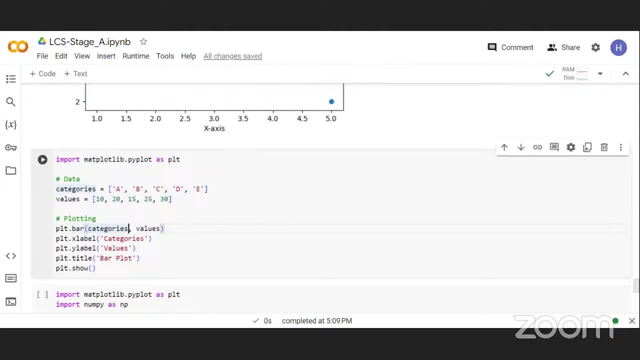 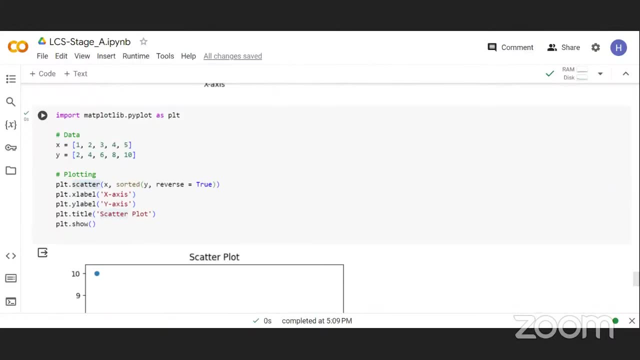 you can provide non-numerical values as the x or y axis. so if you are provided, if you are provided something that contains non-numerical values for these plots, you'd have gotten an error. because for these plots, both your x-axis and your y-axis, they have to be numerical in nature. but when you 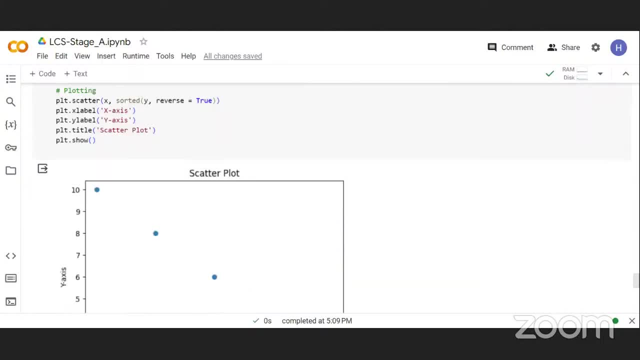 want to try and put a bar chart or something like a pie chart. you can provide non-numerical values and matplotlib will be able to understand that, and you can provide non-numerical values for each plot, so you can set this to be a good plan. so we are going to be using this for 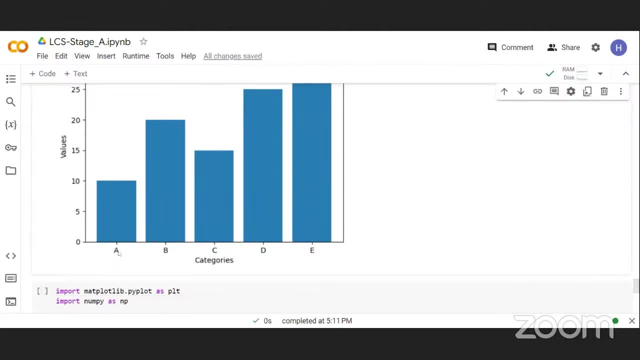 so for the bar a, so for people that fall into category a, there are the number of people fall. stop at 10. but people are falling into category b. um, they get up to 20 people in category c are no more than 15 people in category d. they go as high as 25 and then people in 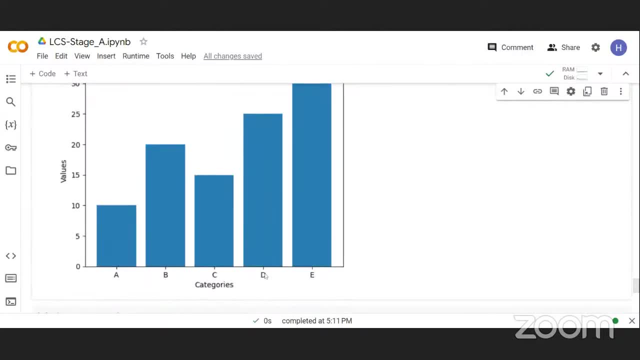 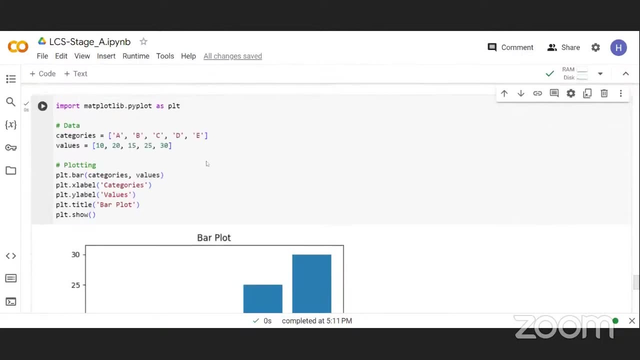 category d are the highest, with a value of about 30. so this i can generate a bad chart that you can use to just um visualize the amount of distribution that each of us will get and if you are doing the same thing for the other ones, you can directly select the. different ones. you can give them the same value as much as you want, and then, if we select the different ones, we get the same value. so we are already taking the same value in the other ones. we're getting the same value of the other ones. so this is actually. 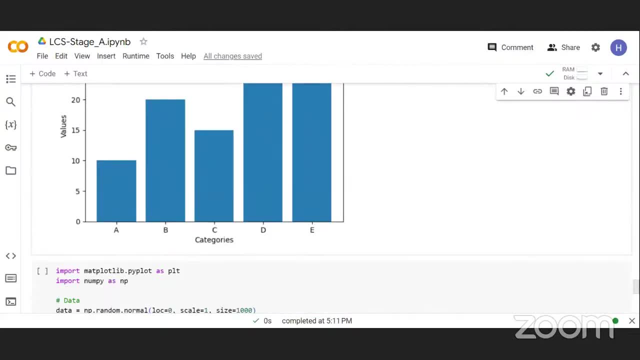 that each unique category falls into for a data set when you're trying to visualize it, When you're trying to visualize distribution. so the most times when you're going to make use of a blood plot, most times is when you're probably trying to show the count. 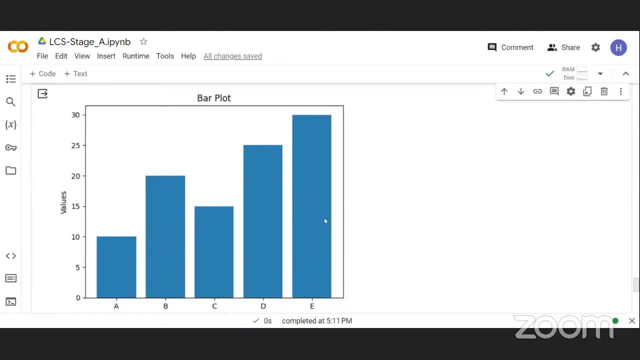 So if you're trying to show the amount of data set, let's say something like a gender column in your data, and then you want to show the different people that fall into the different genders in your data set. all you just have to do is to count the values in that category. 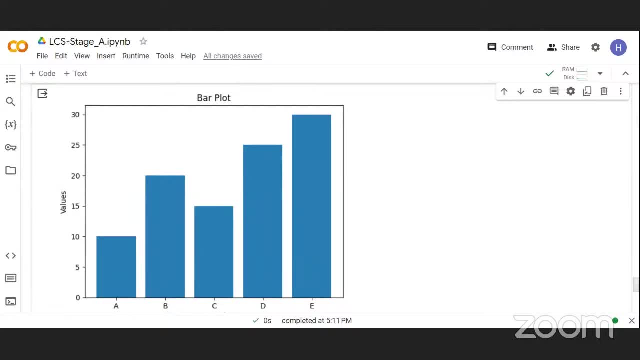 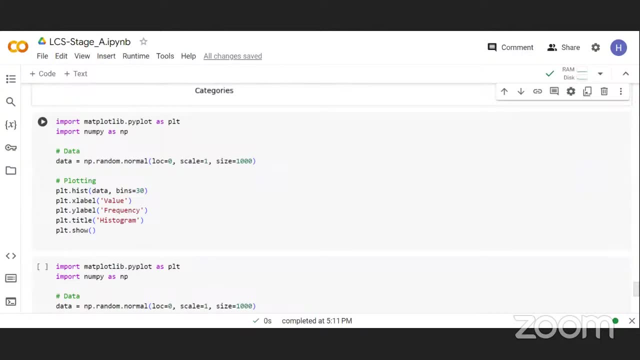 and then plot it And then you can show the different values in that category. So the next thing that we're going to be showing is an histogram. So an histogram is almost the same as a bar chart, but the histogram just gives us a data set in different things. 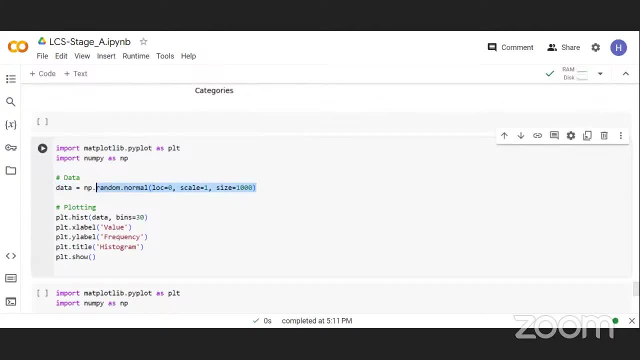 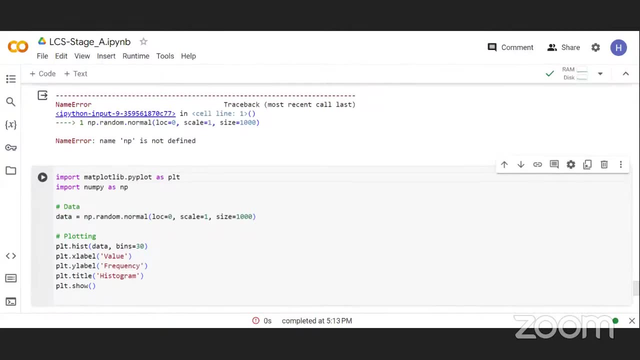 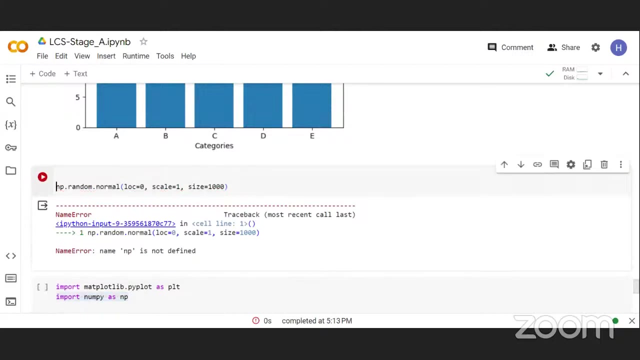 So before I show you the histogram, let me just run this code here. Let me run it separately. So if you want this code, okay, I've now imported NumPy. Let me import NumPy. Let me import NumPy as np. 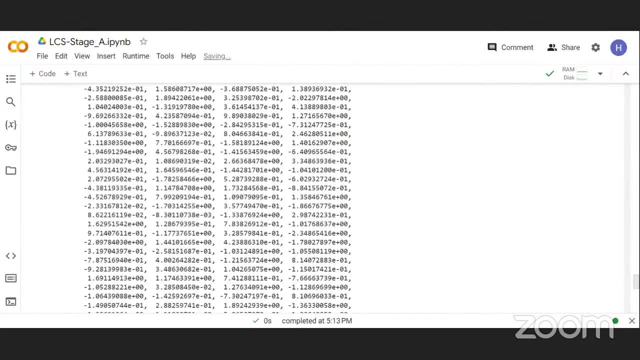 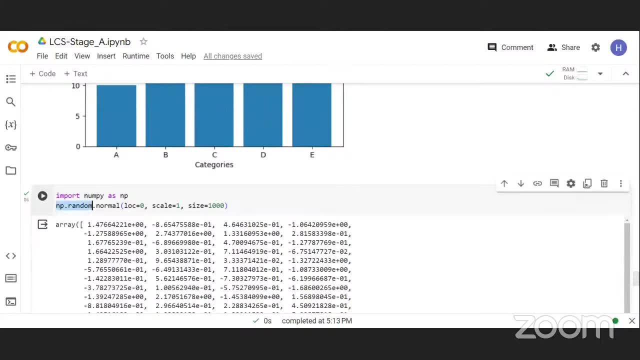 So after importing NumPy as np, so this code here is giving me what? Well, this is quite a lot of values. So what this does is it gives a random normal distribution. So for people that are familiar with mathematical or statistical terms, 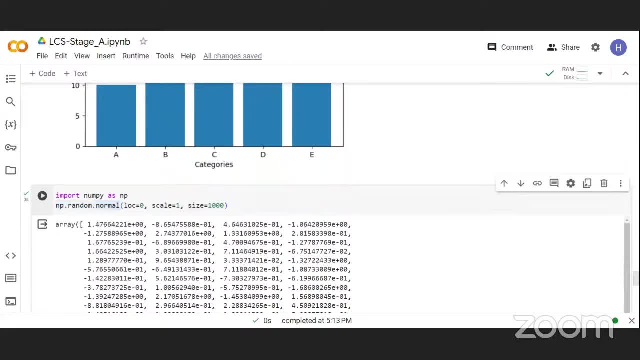 so this is a random normal distribution where the mean is equal to zero And then the standard division is equal to one. So what a random normal distribution is a statistical probability that tries to when you sum up the values in the array and you divide it by the number of values there. 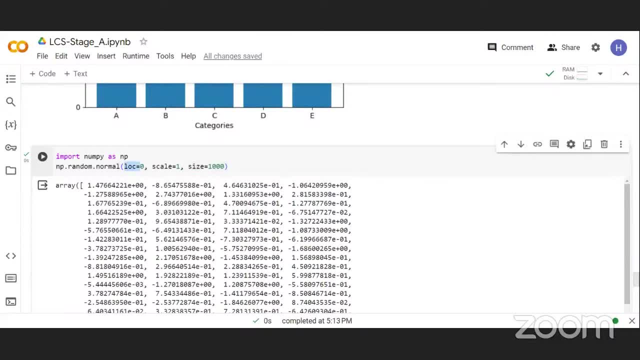 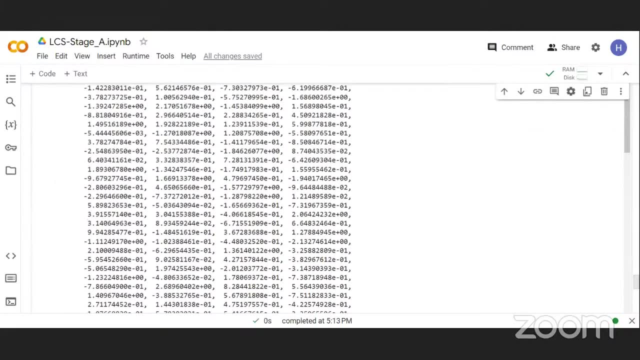 you should have whatever you provide as the LOC. That's the location, which is the mean, And when you compute the standard division, you are going to have the value you have as the scale. So this is quite a lot of values. These are 1,000 different values. 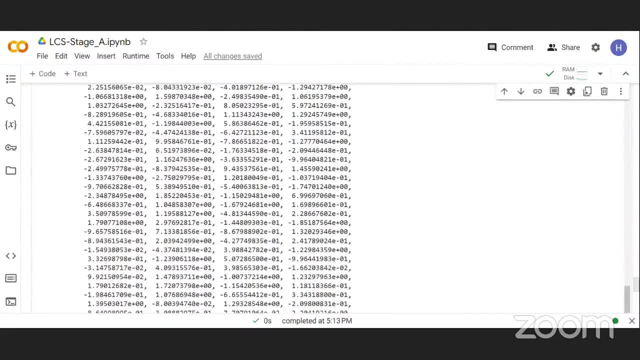 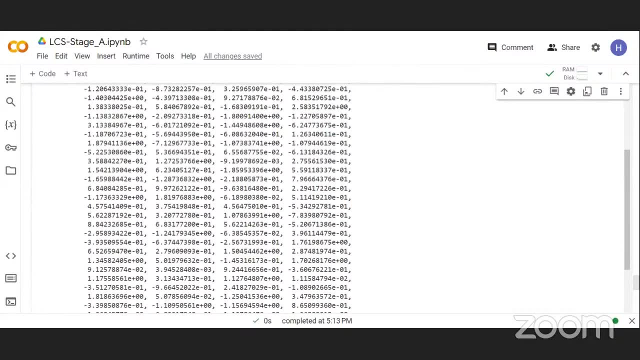 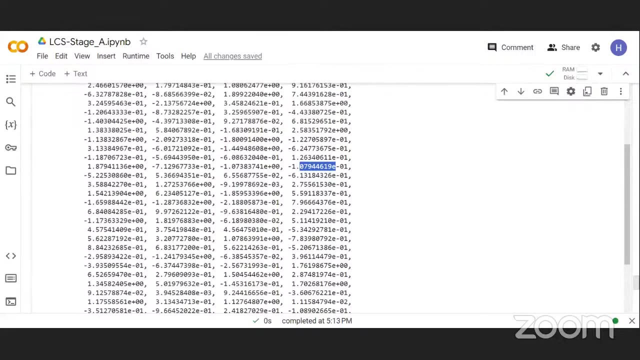 So imagine you are trying to and for these kind of values. now something like this is very rare that a value is going to occur twice in this kind of scenario, because this is a lot of different values with a lot of decimal points. So at least there will be one decimal point that will make another value. 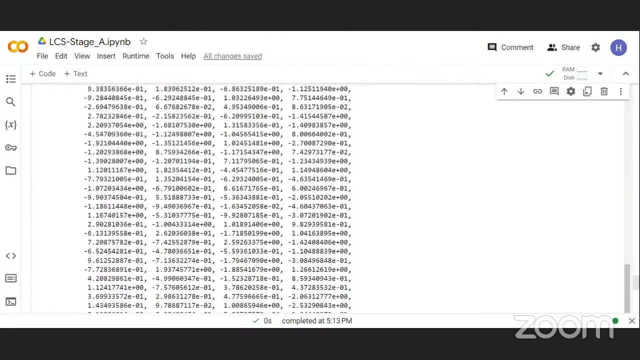 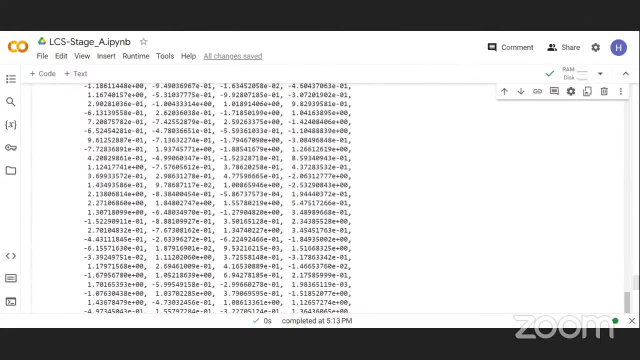 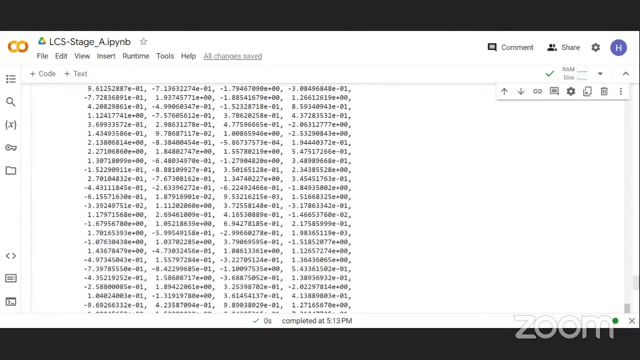 very, very different from another. So in a case like this, where you have a data set with a different array of random numbers, where you know that it is very rare for two numbers to repeat itself, So in this kind of thing we call this kind of data- 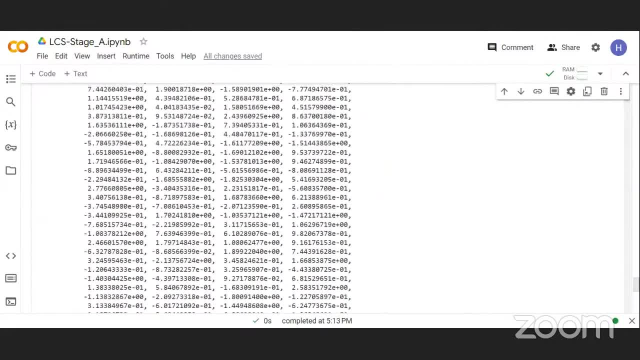 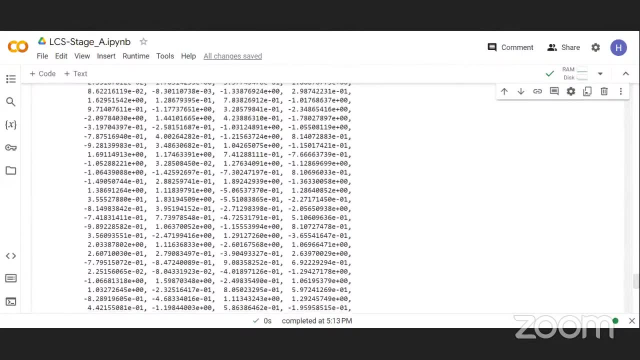 we call them numerical data or ordinal data, So these are data sets. This kind of data is a data where it deals with numbers that cannot be repeated, It's not categorical in nature. So this kind of data, the easiest way to plot this kind of data, is using a histogram. 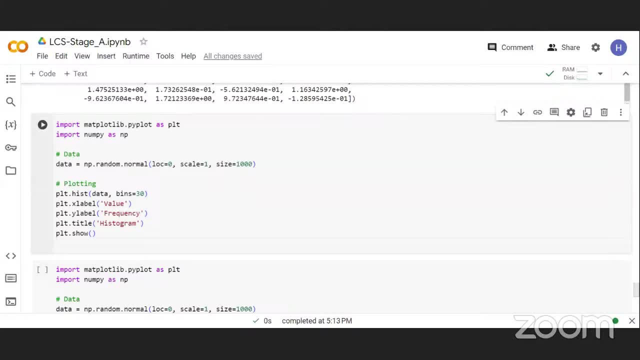 So all you just have to do is: okay for these values. I know these values are quite large. Let me take them in groups, So you can take values in groups of 10.. You can take values in groups of 20.. 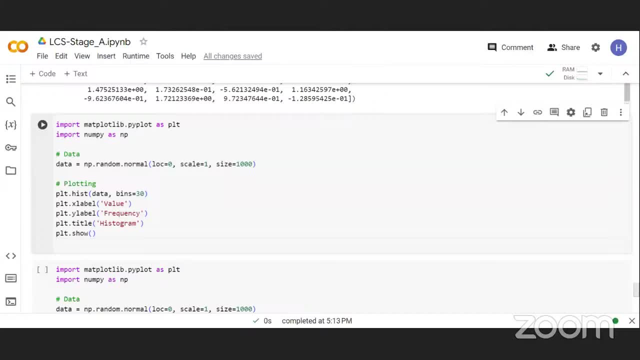 You can take values in groups of 30, depending on however you see fit, And then you can plot it using a histogram. So when you create an histogram, all you just have to do is to pass in all of the different values that you want to plot. 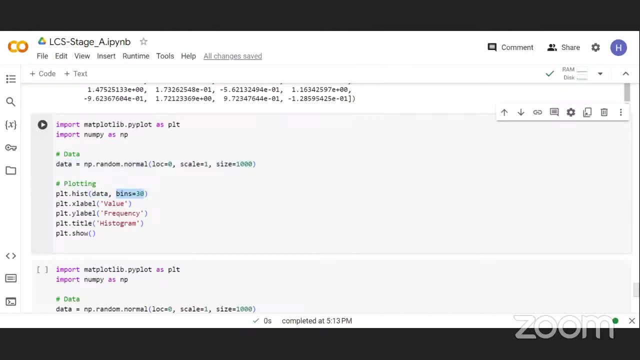 So mark, plot, leave. and then you have to provide the bins. So the bins gives you the, what The bins gives you the number of groups that you want to plot. You want to take it in. So mark, plot, leave is smart enough to get the highest number. 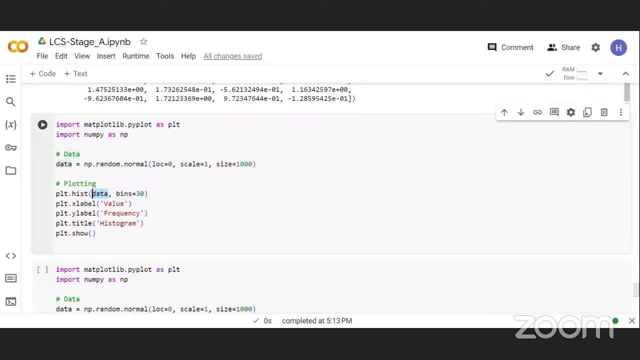 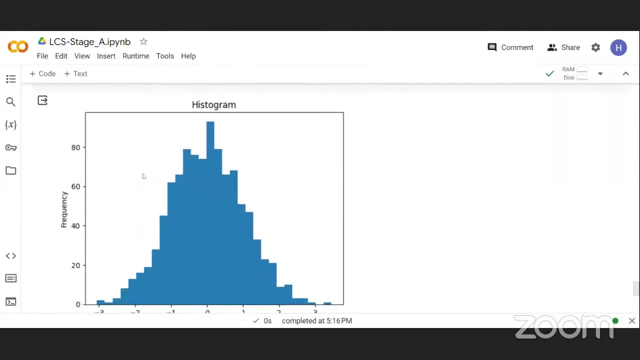 and then get the lowest number from this set of values And then for every value that falls into the different categories, for whatever you provide there, it will create an histogram that shows you all of this. So if you want this cell now, so this is the histogram. 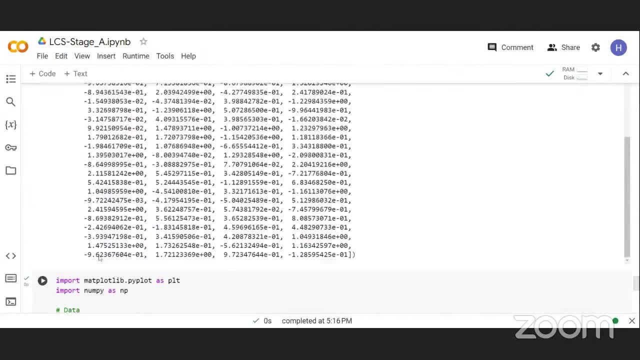 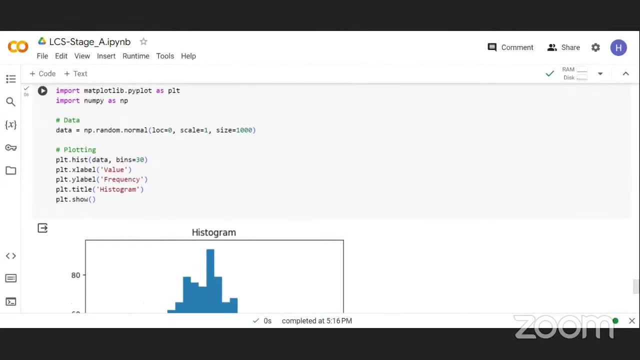 And you can see that the minimum value so for this data, for this set now, the minimum value is minus three. The maximum value is two, And then different values there in the bins. So we have minus three to three And if you try and count this, 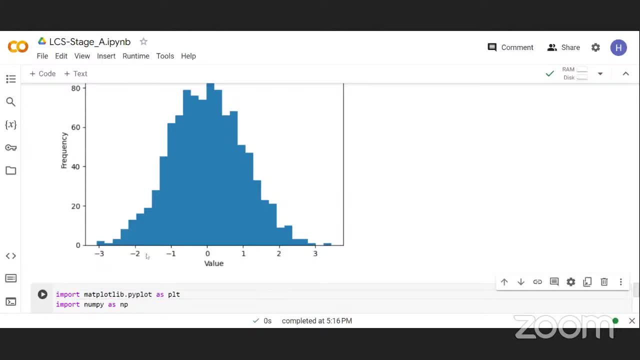 this is probably going to be like this: one, two, three, four, five and six, So this is five bins And it has been able to like divide all of the values that are here, this 1000 values, to try and show us. 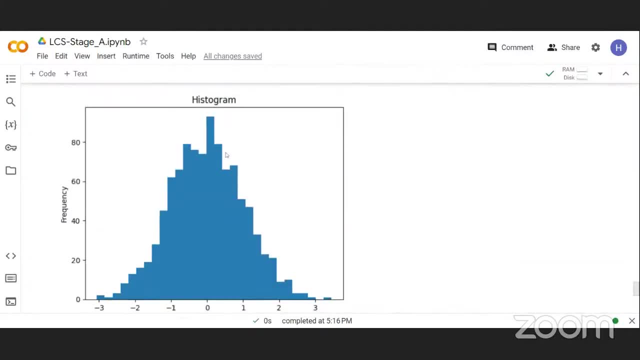 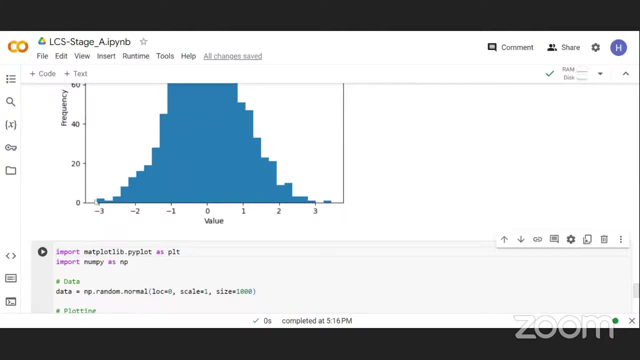 okay, for these different ranges, these are the values that are present in the data sets. So you can see, from minus three to three, the range of values that show. they show and you can see that if you are very, if you are conversant with statistics and distribution. 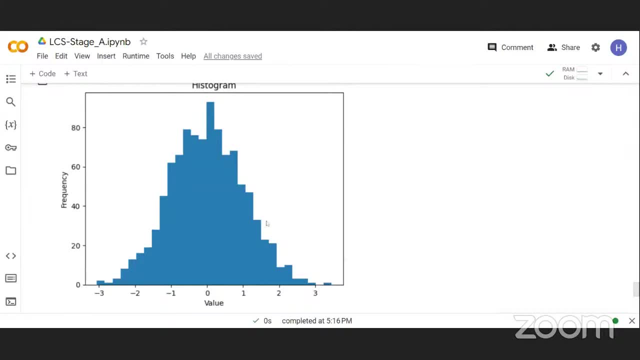 a normal distribution always has a bell-like shape, a bell-like shape And if you try and plot, if you try and take a curve around each of these edges, you'll see that what you'll be having in the end is going to look. 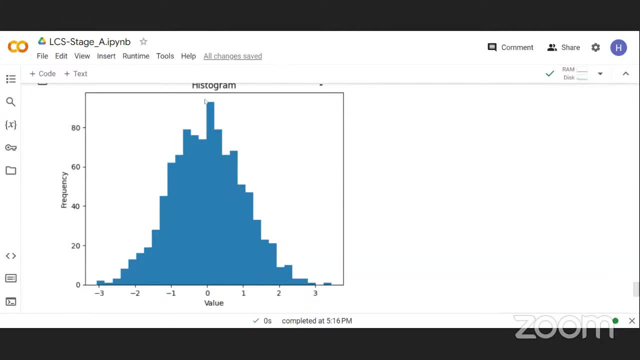 is going to be shaped like a bell, And this is sometimes when you can just plot a histogram or plot a logarithmic distribution to just know if your data sets are normal, if they are normal. So based on this, you can know if they are skewed or not. 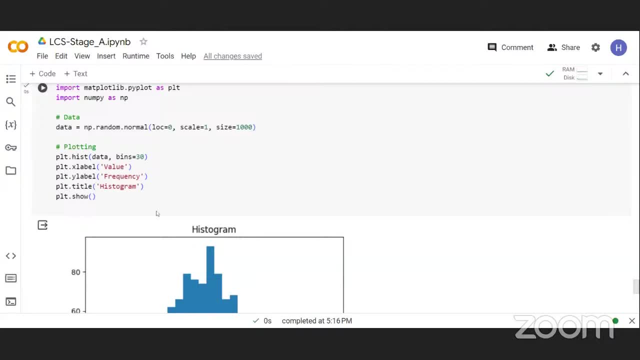 But we'll talk more about that in the next stage when you start taking live coding sessions for that stage. But that's a very good introduction. So this is a histogram. So a range of values are four between minus one and zero around this range. 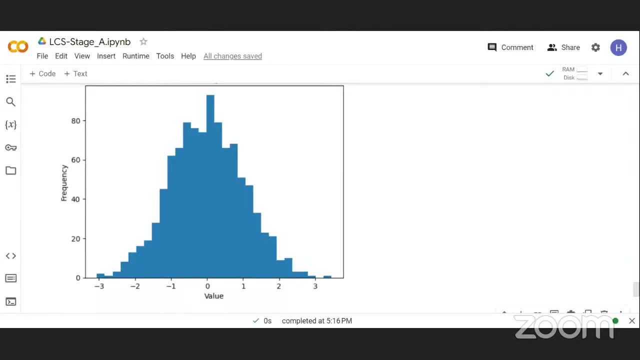 and then that looks like the histogram. So you have different customizations where you might not want your histogram to be mumbled up together like this. You might want each bar for each histogram to be separate, And then that's one of the ways that you can visualize your data. 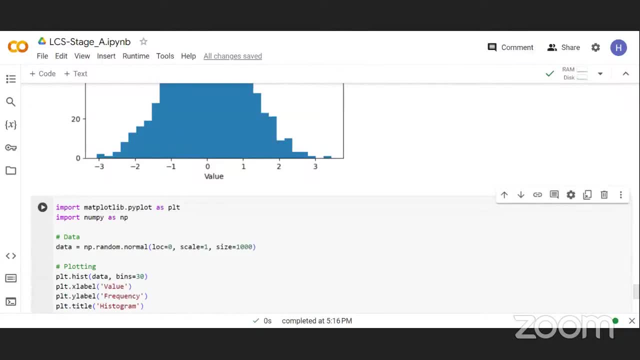 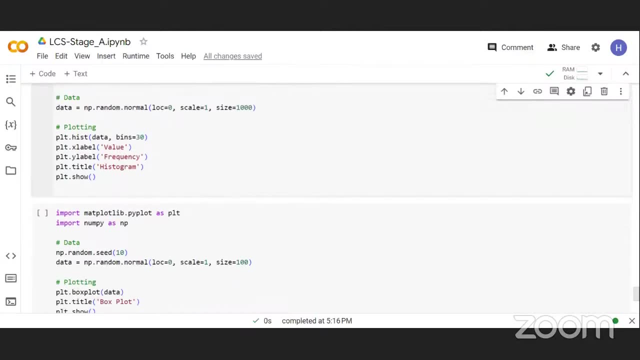 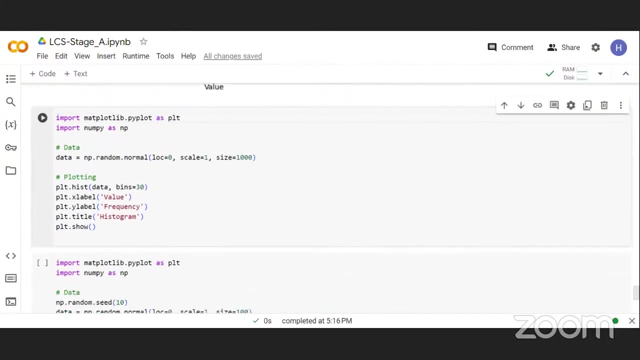 Another plot that I'm going to try and show. okay, I think this is the same plot for Instagram. So another very, very popular plot is a pie chart. A pie chart- Okay, I don't think I have that of a pie chart here. 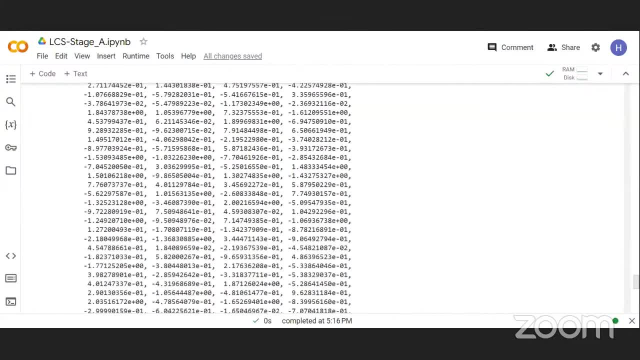 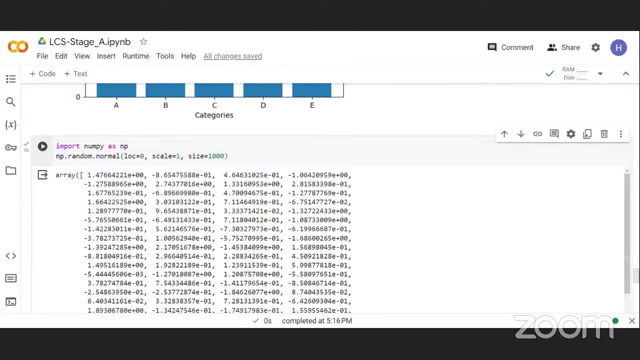 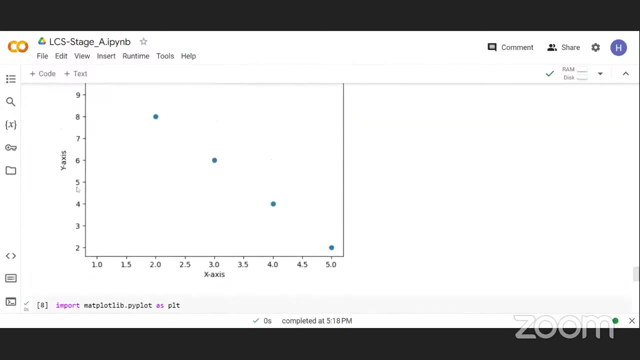 A pie chart. It should be somewhere around here. Sorry, let me just clear this. Come on, Let me just clear this here. Oh, let's see, Exactly. So just before this bar plot here you should also be able to create. 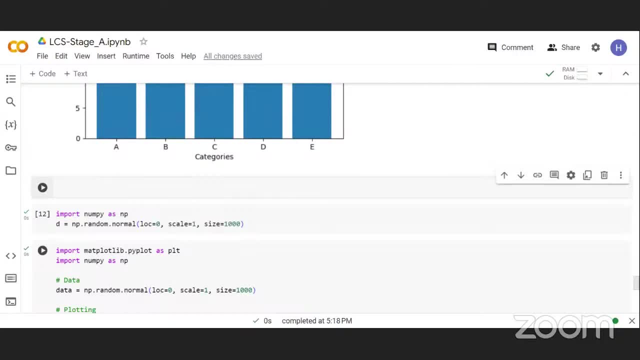 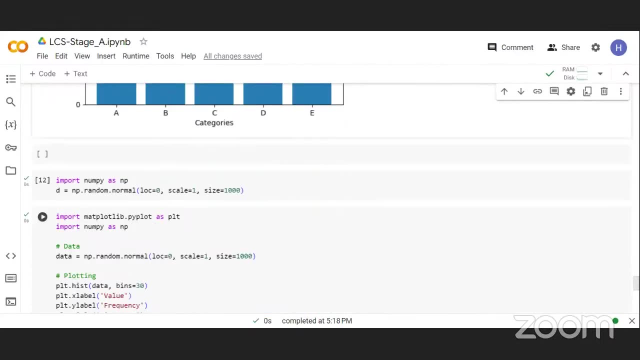 you'll be able to create a pie chart. So to create a pie chart, I'm just going to like it's basically. it's basically what I did for the bar chart. I'll take this, I'll copy and paste these values here also. 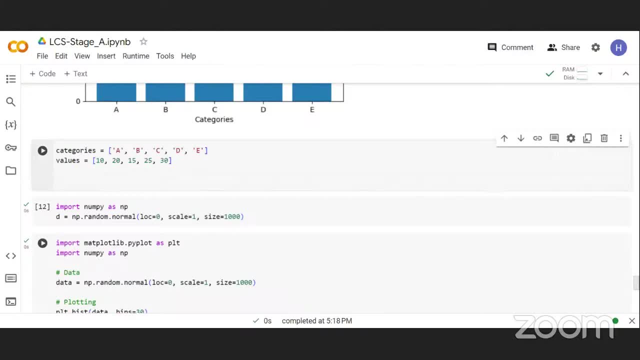 But now, instead of doing plot dots bar, I'm going to do plot dot pie. So when I do a plot dot pie, I'm going to say that: okay, the labels. I'm going to say that the labels are the values. 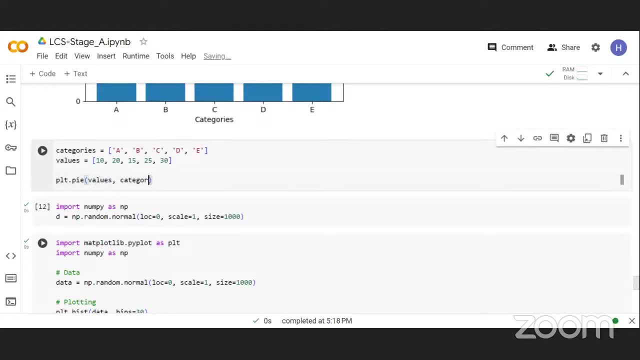 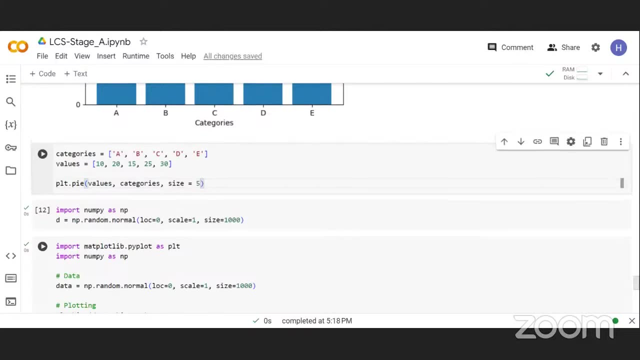 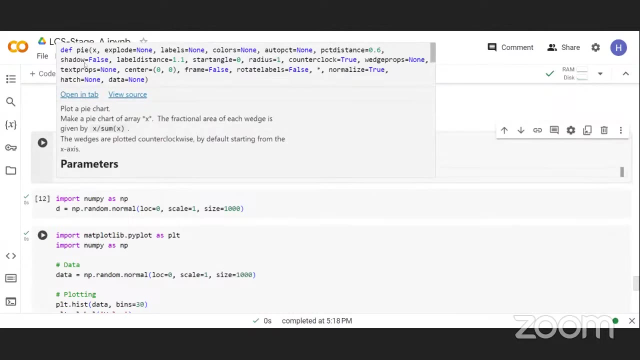 And then categories, And then give me the size to be close to five. So with this now, rather than what you have for your bar charts, you can see, even if you just try and stay here, if this comes, I can see this is the pie. 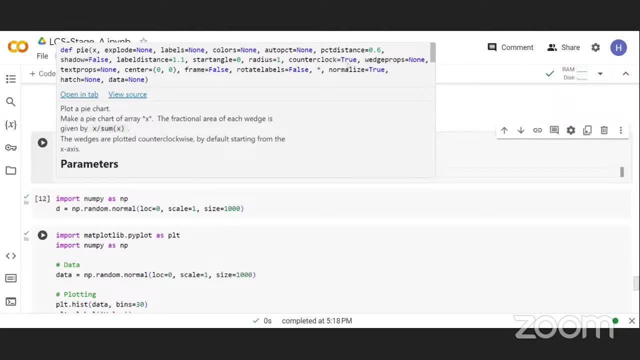 So you have a lot of different, a lot of different options that you have for your pie charts. Okay, Pie chart: explode is equals to none. Data is equals to none. Blah, blah, blah. Labels: Blah, blah, blah. 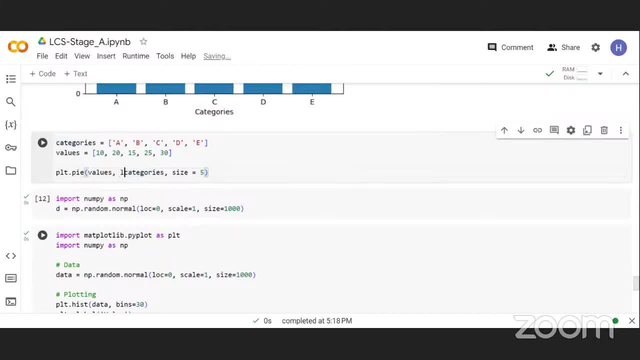 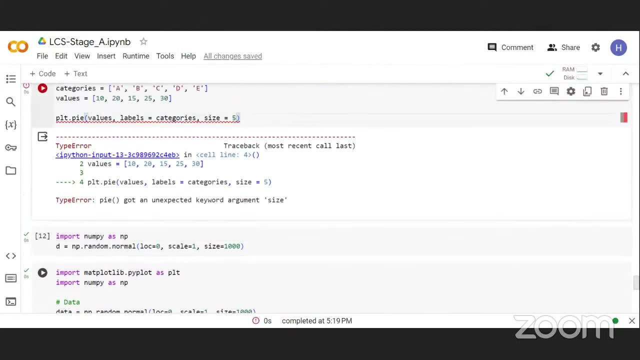 So this is just me saying that, okay, set the labels. So, because of categories. so if we try and plot this now, okay, that size, let me take away the size variable. So let me plot this. You can see that. 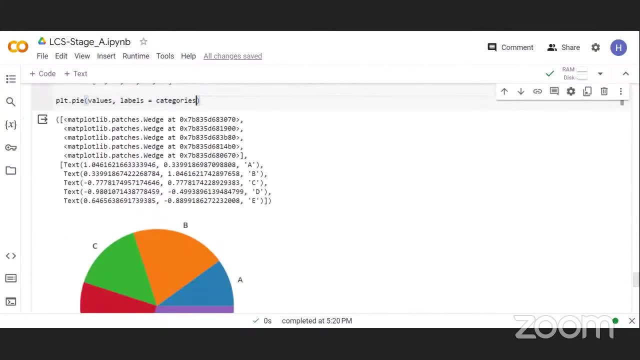 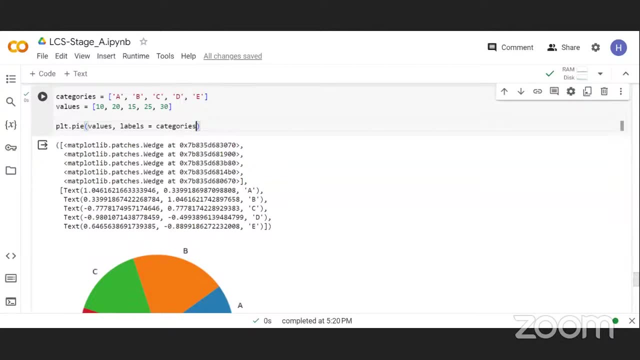 this is the pie chart, So for A. so what he tries to do is he tries to show you all of this in a pie chart. So we have five values: A, B, C, D, E and E. We have five values of A, B, C, D and E. 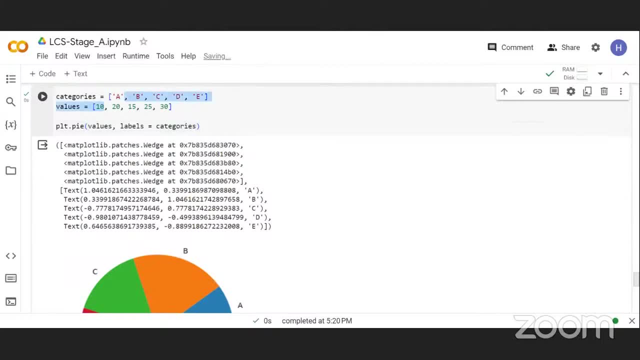 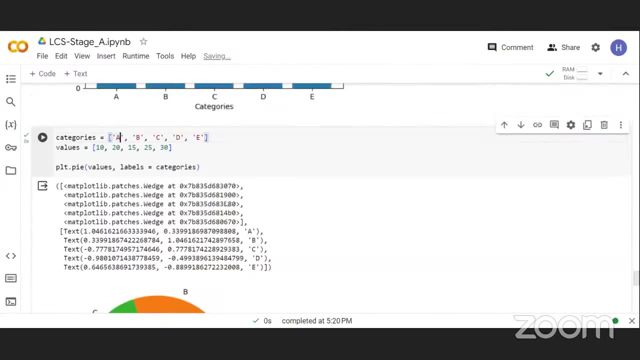 And then for A we can say: the value of A corresponds to 10% of the data. So you can see, A is the smallest pie, We just 10%. We can even make this right: the value for whatever it's meant to write there. 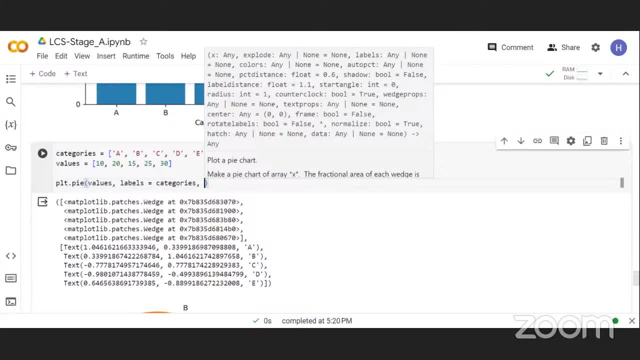 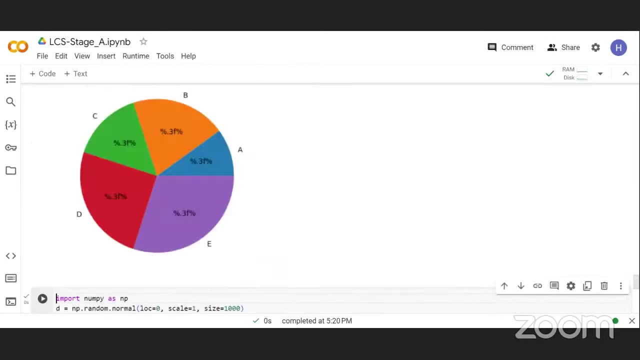 And I think it should be auto PCT, Auto PCT, And then you format it with dot two F. I think I think this one should be one, So it's in complete format. Let me try it one percent on the back. 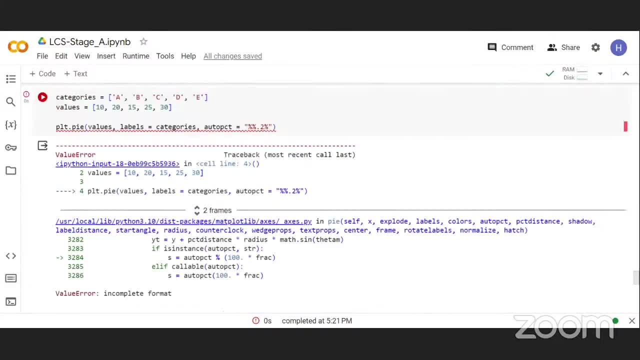 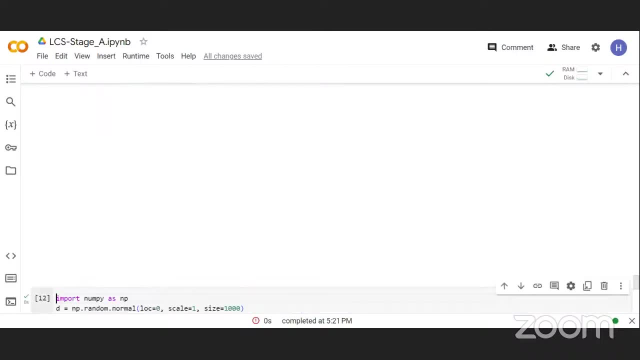 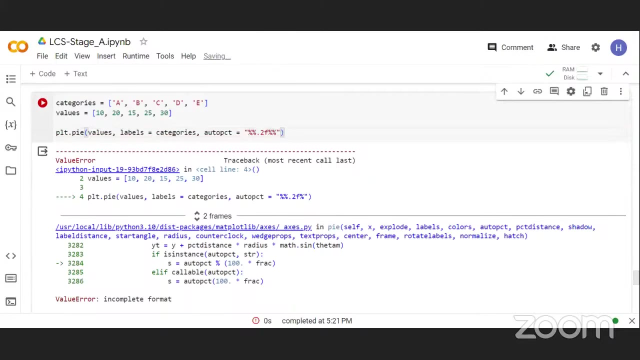 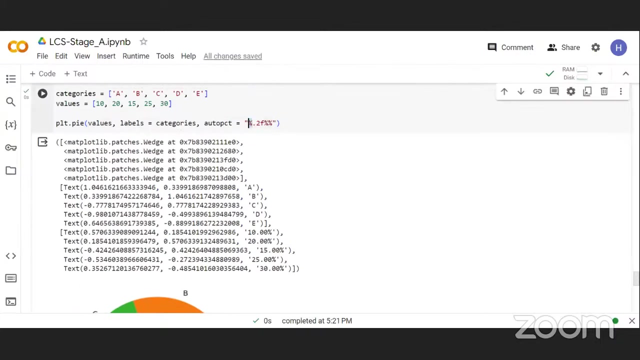 And two I will get. let's see Which one is meant to be: two percentage. There's all the formats, this thing When you want to write the percentage of exactly. So this is the correct format. So you have one percentage in front. 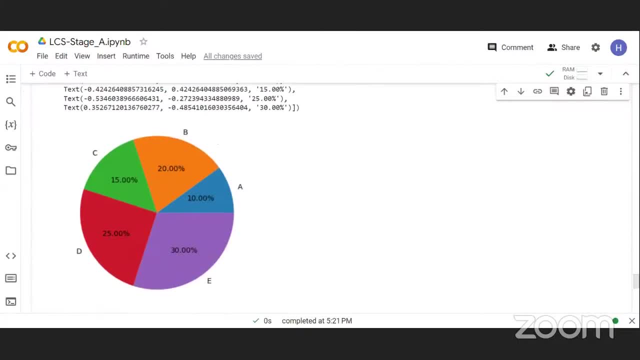 and then two percentage below. So you can see that what this is trying to do. now this is: if you calculate this, 25 plus 15 is 40,, 30 plus 20 plus 10.. So this is like 100%. 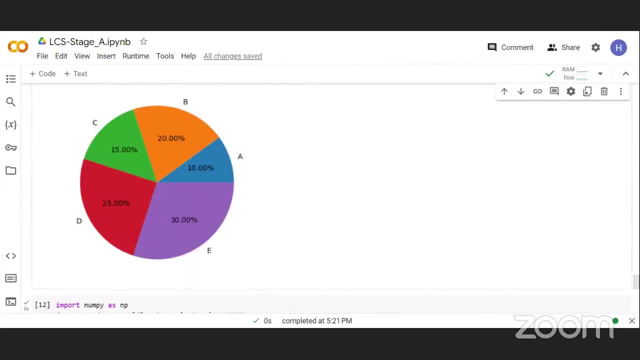 So you can't have a pie chart that is more than 100%. So what we are trying to do here is okay for category A. category A takes 10% of this data frame And then A just has a 10% aspect of this pie chart. 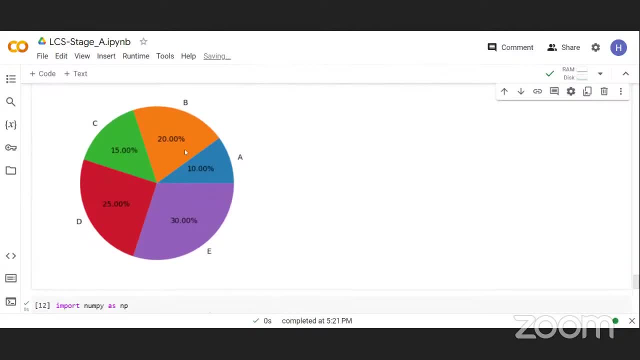 And then we have category B. Category B has what? 20%. Then we have category C with 15%, and category C here is 15%. So these are. you can plot a pie chart. Either you can plot a pie chart. 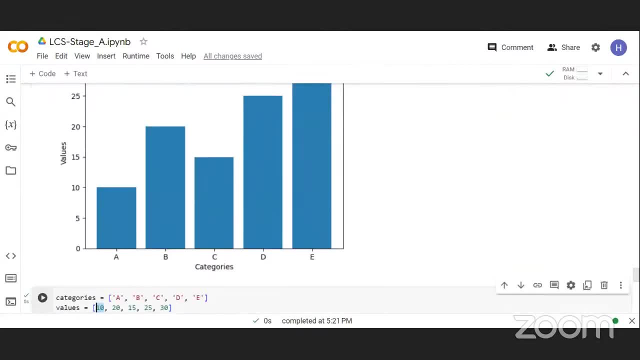 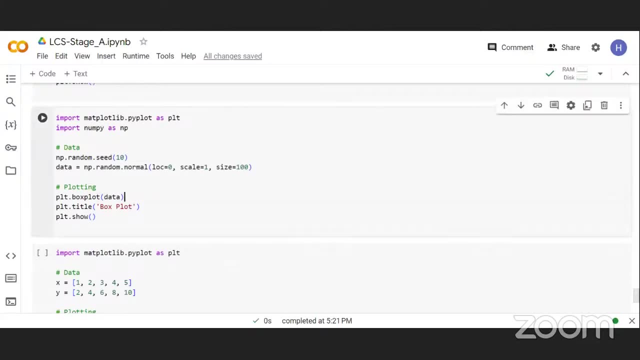 or you can plot a pie chart where you give different percentage for each of the values. So this is just a basic, very, very basic. So we have spoken on Instagram- Instagram, sorry. So the next one that we are going to be showcasing is a box plot. 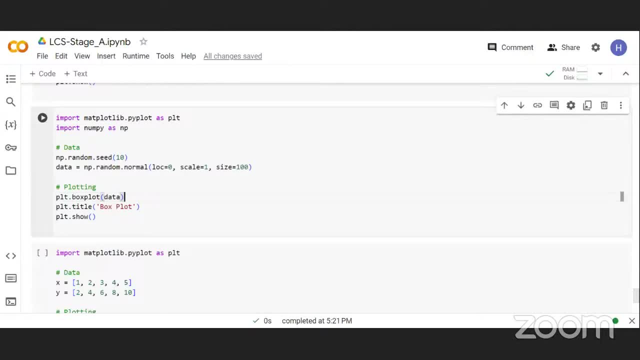 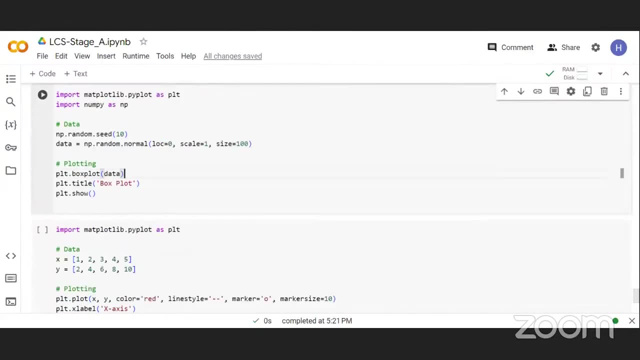 So what a box plot tries to do is it tries to give you, rather than give you, the distribution of the data using an Instagram. it tries to put all of them into one single rectangle. So one of the very, very best use cases for box plots is to showcase 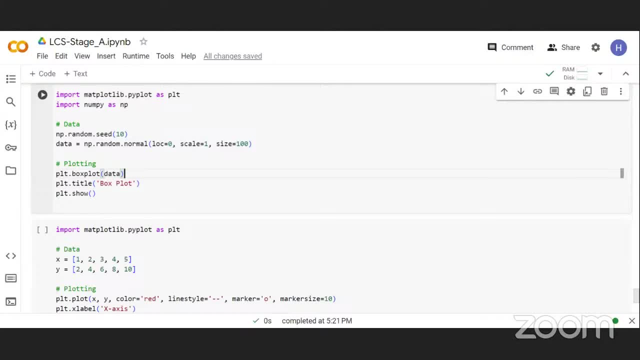 um outliers in the data. So over time, as you begin to go into data science and stuff, you'll see that box plots will be one of the plots that you'll be using a lot, because you'll be using box plots to check if your data set has something that we call. 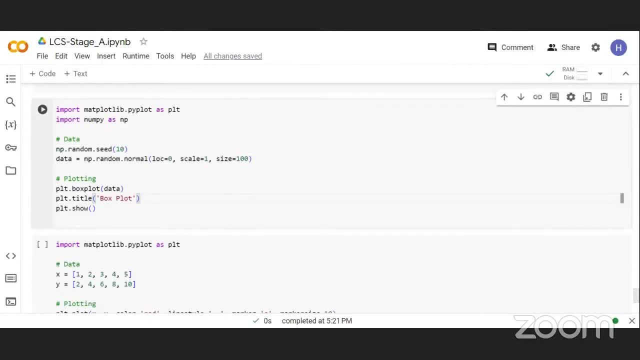 outliers. So outliers are um. outliers are values in the data set that are very, very far away from the normal range of values that you can see in the data sets. So you can see this is just creating the um. 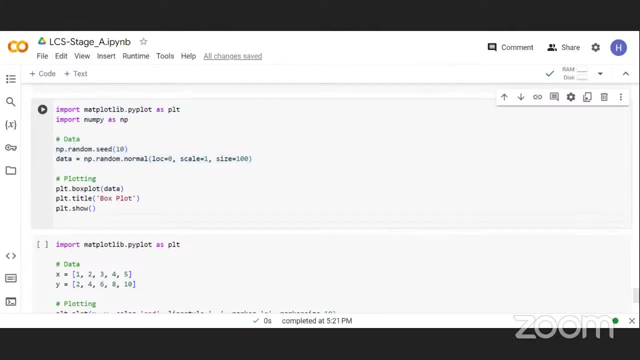 same data sets, that, the same data that we did for the pie charts, this program. sorry, But now let us try to see it in a box plot. So this is the box plot here. So you can see in this box plot. 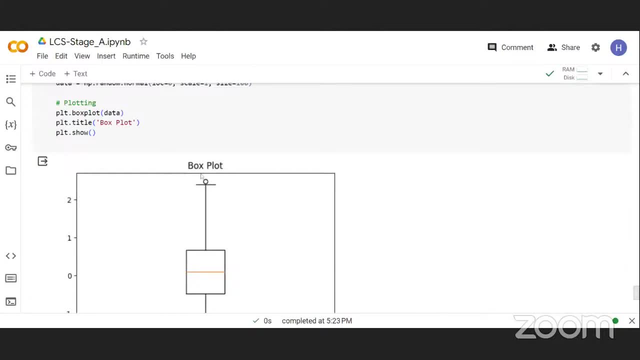 what this value here. so any value that comes above this line here in the box plot shows that this is an outlier. So this value is too much, is very, very much far away from most of the values in these data sets occur in this box here. 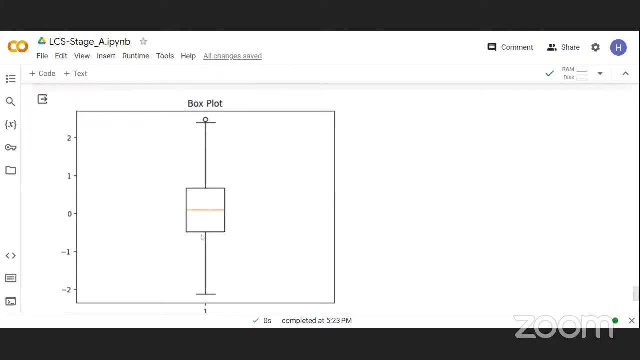 So we have some values that go up all the way here, Some values that come down up the way to minus two. So you can see that this minus three that we had there is, um, almost an outlier, because even in this value here, 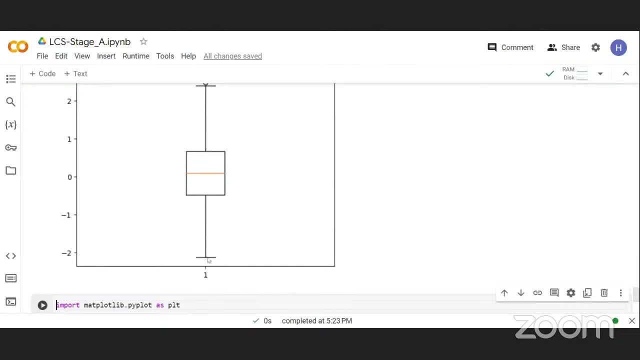 it just stops at minus two, And then there's a value somewhere around here that's at minus three, And then you can see this histogram: after this stopped at three, there was another value that was even away from this point of three, this small value here that you can see here. 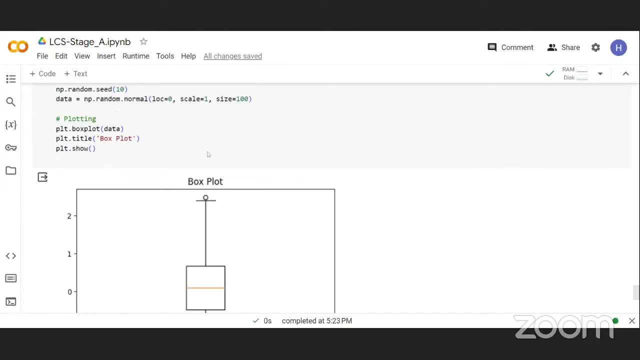 That is what this dot here is trying to show: That there's a value here that is very, very much far away from the range of values that are what's popular in this data set distribution. So that is what you use a box plot for. 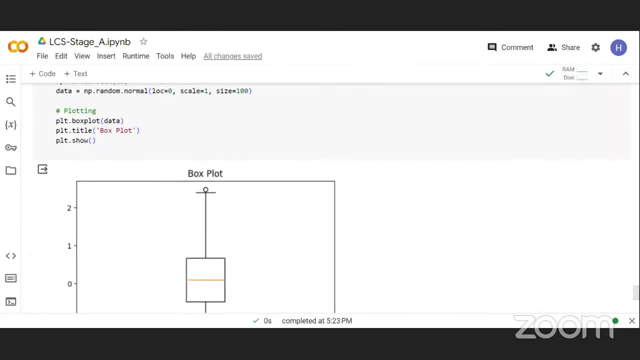 And there are ways when you want to check if your data set has outlier, because one of the things that you must deal with as a data analyst or a data scientist, when you are trying to analyze your data, is outliers, because outliers have a way of changing the inference you are making. 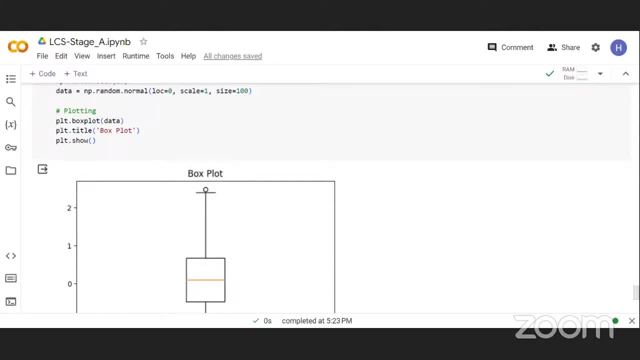 One very quick example of what an outlier is. So let's say, in a locality, most houses or apartments there are being sold at around 20,000 or 25,000.. But then something happened on a particular day, Let's say the owner of the house died, or they found that gold can be mined in that particular house. 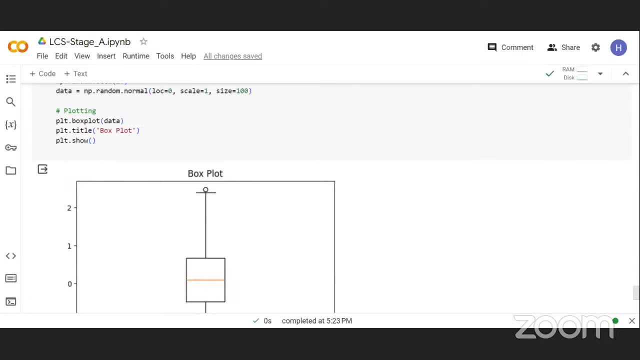 And then the house got sold for around 150, rather than the normal range of values, Or 20 to 25,000.. So when you are trying to compute data, if you are trying to calculate the mean, for example, let me just try and probably try and showcase something like that here. 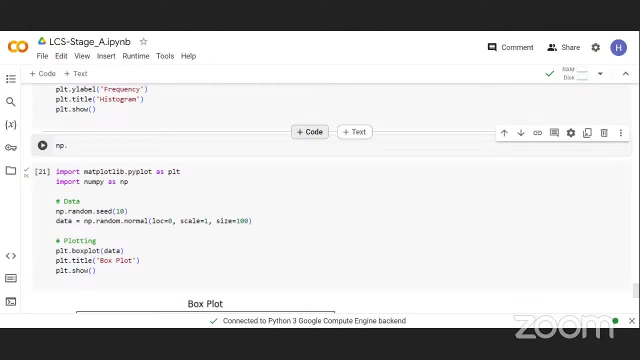 So let's say I want to do MP dot mean. Okay, We have in that locality. houses are being sold at 20 naira or 22 naira. We have 23.. Go back to 20.. Go back to 25.. 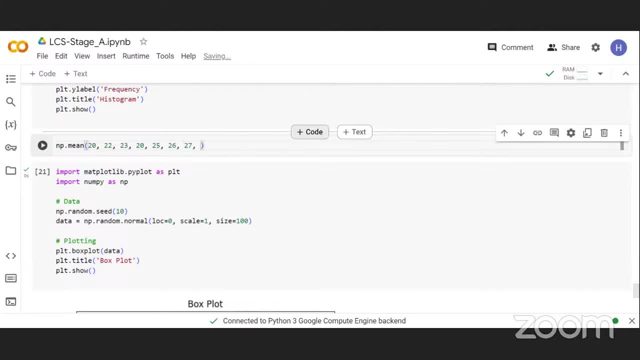 Okay, Go back to 26.. Go back to 27.. Then we come back to 22.. Then we come back to 23.. Come back to 24. Like that. So let's say these are the ranges of values of houses. 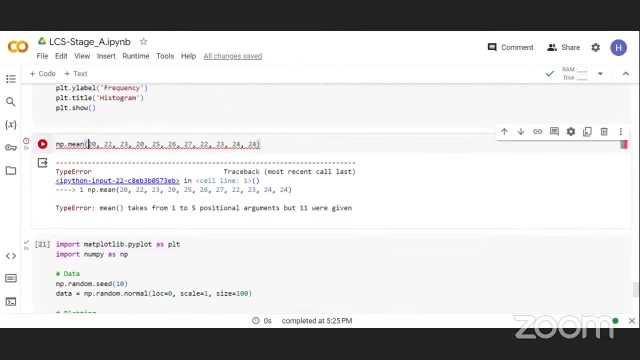 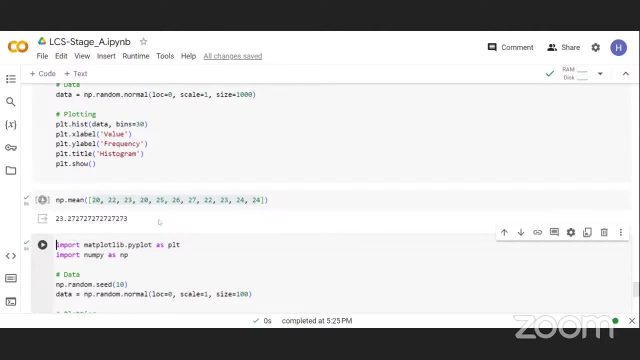 So if you check this mean- Oh sorry, This is meant to be in a list. So if you take this mean, you see that, okay, the mean is also in between the frequency and the values, that we can say It's 23.2.. 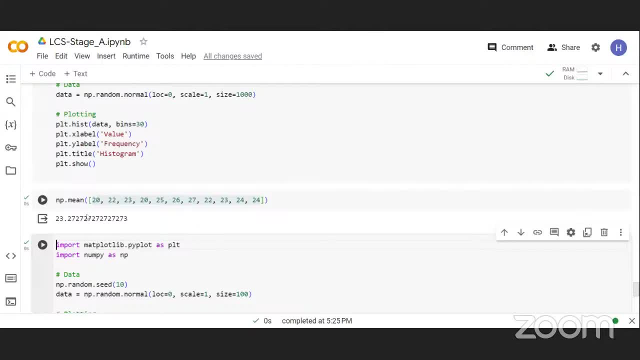 All right. So when you go to a locality and you try to calculate the mean of the price of the different houses, you can see these values. It makes sense. But imagine that this particular house, on the day it was being sold, it was not found out that this sold. 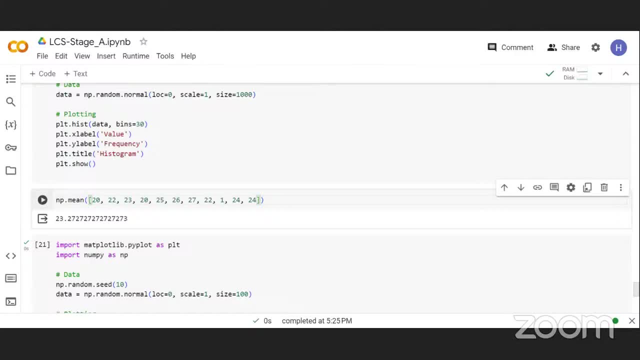 this house has something like gold in it. So instead of it to be sold at 23 naira, normally they want to sell it at 1,000.. And it got bought. If we now try and calculate the mean of this particular value, 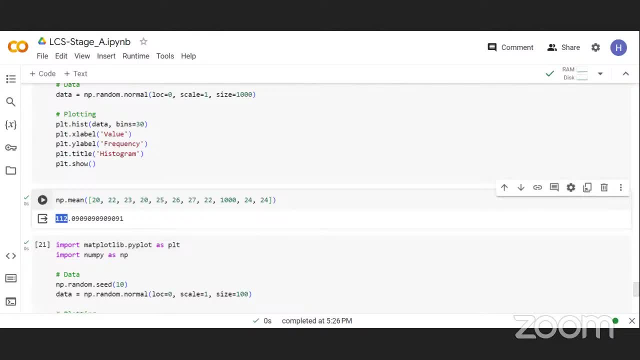 see where the mean is the 112,, which is very, very, very far away from the normal values of 20, 22,, where every other house in the data set is going to be sold in. So this is what appliers can do to your data. 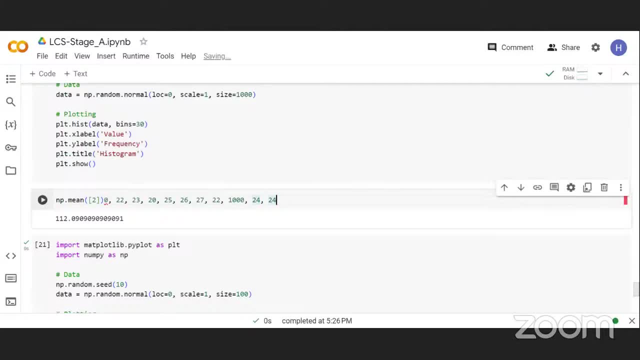 An applier that is to the right side drag your mean very much far away from the normal range of values that you should have. An applier that is on the left side would drag your mean very much lower than the value that it should be. 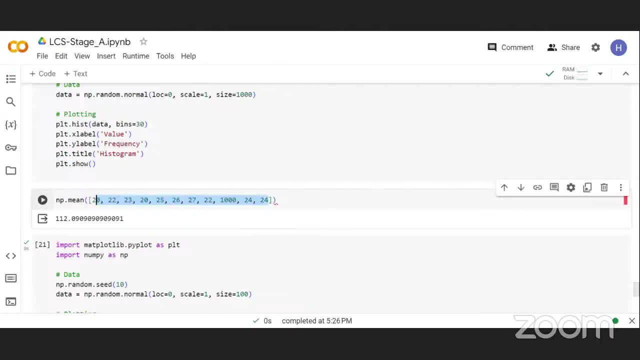 So one thing you should do so that you won't be making the wrong inference. So imagine you were analyzing the data and then you just make an inference that, okay, we can. we can confidently say that houses in this range have a mean price of 102,000. And then people now go to the locality and start saying that houses here are just being sold at 20, 25,000.. It was only one house that got sold at 1,000 naira And that was because it happened because of this particular factor. 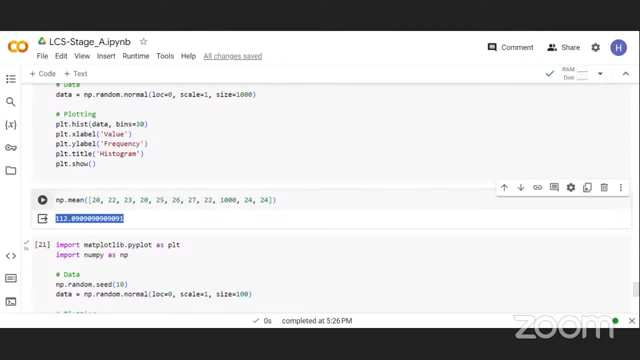 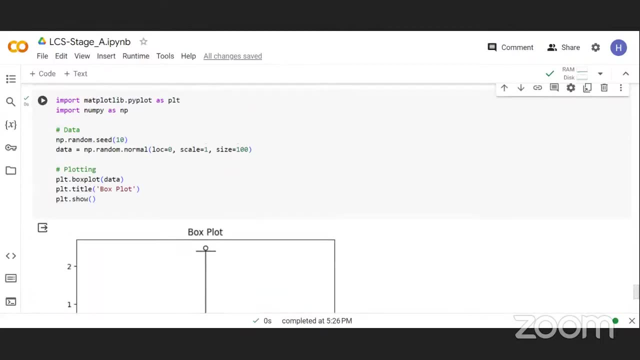 that was not captured in the data set. You have already made the wrong inference because you did not take account of the applier that showcasing your data. So a box plot is one of the ways that you can try and you can try and visualize. 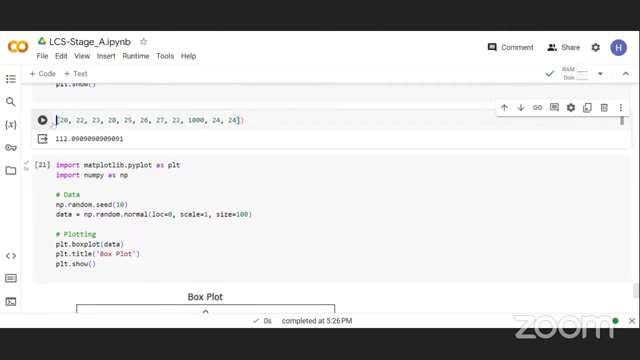 If I try and visualize this now using a box plot, let me say plcboxplot, Okay, And let me try and show this So you can see that it is showing the ranges of values that we have here. See where these values are. 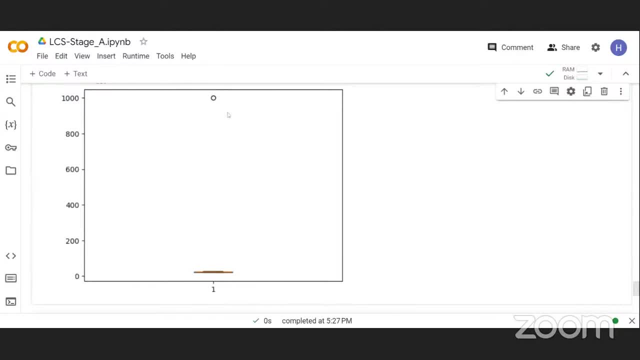 But then we have an applier that is showing that it's very, very far away from this address. So any inference you try to make using this data this way, this will be wrong, because that applier is taking you away from the actual inference. 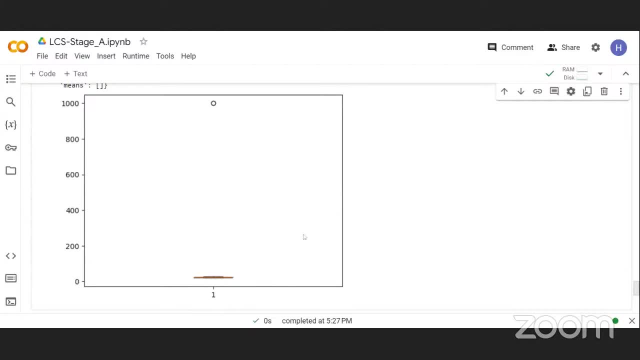 Because when we are making all of this inference or statistical assumptions, we are trying to do it Okay When you take a random sample, when you take a random sample at least 20 out of 30 or 24, like at least 20 out of 25,. 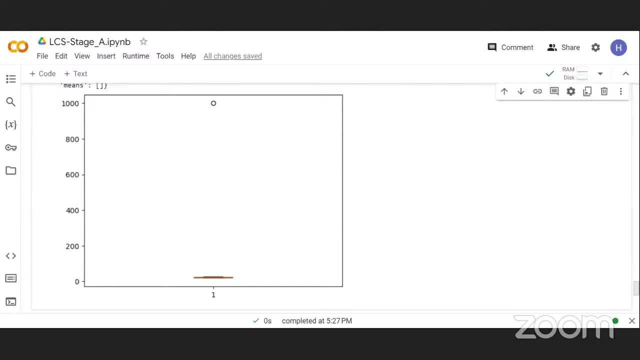 20 out of 30 should follow 20 out of 25 should follow the. 20 out of 25 should follow the should follow the inference that you are making for whatever it is that you are doing, So if you have a data that has a lot of appliers in it. 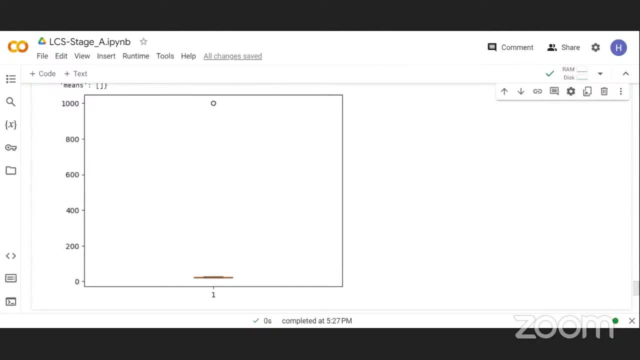 it would be hard for you to make correct inference, because that data, the applier, would just basically take your value away from the ranges of values that you should have. So that's what an applier can do to your data set and you should always try and avoid it. 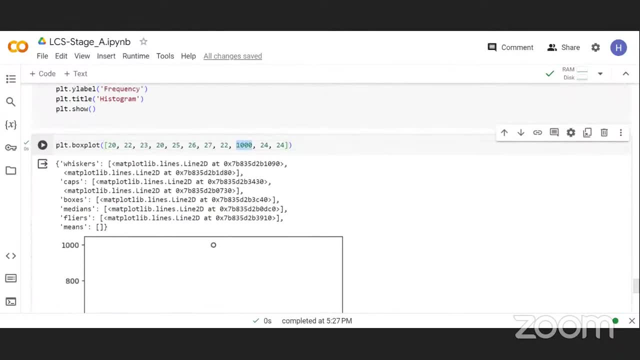 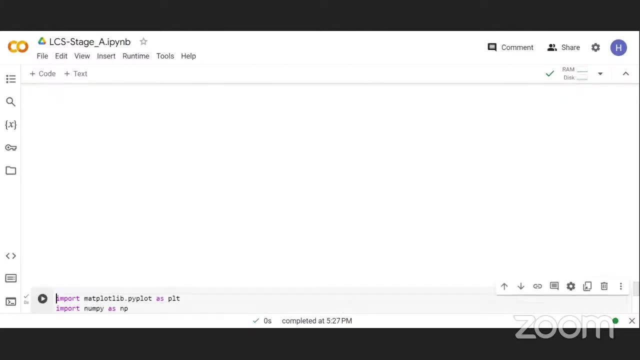 So, but if you try and just remove this applier now, okay, let me control Y, Let me just take away this applier of 1000 and then plot this box. plot. You see that you can see your box plot is bigger. 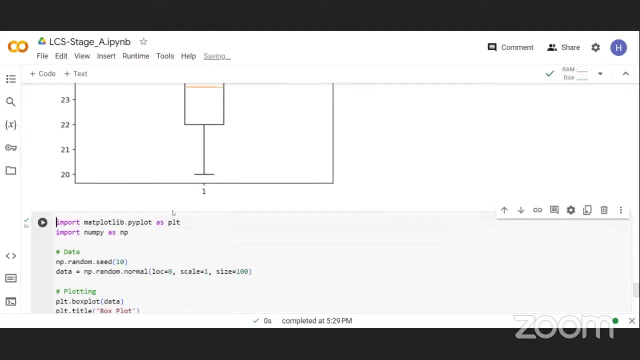 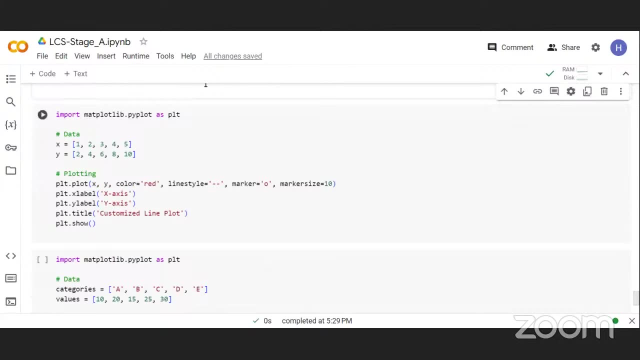 and because this is actually a confident range of values where your data set falls into for this particular range. So that's what you use a box plot for And over time you continue to use it more as you go through a lot of different visualizations and stuff. 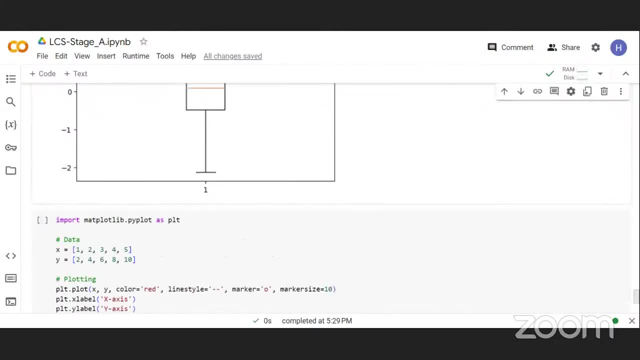 So now I want to show some kind of customizations that you have. So, with smartplotlib, there are some customizations that you have where you can begin to like change how your plot is going to be returned, Because you can see most of the plots that are being returned. 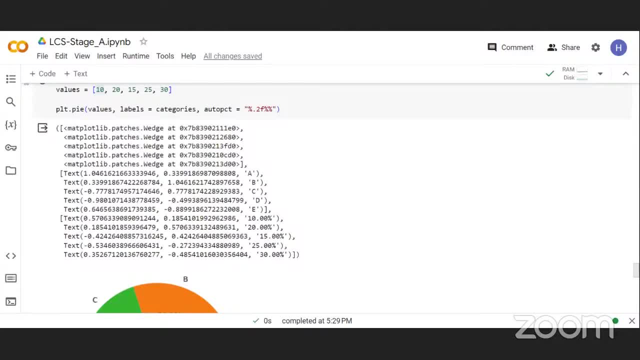 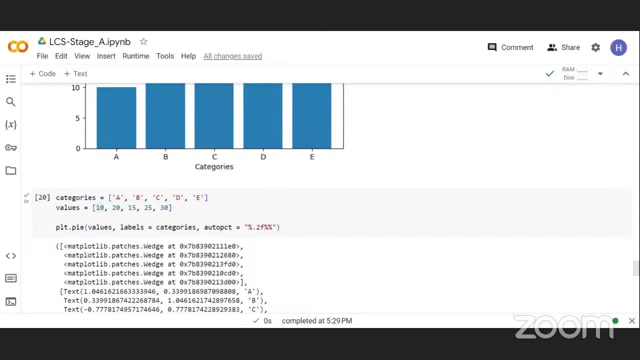 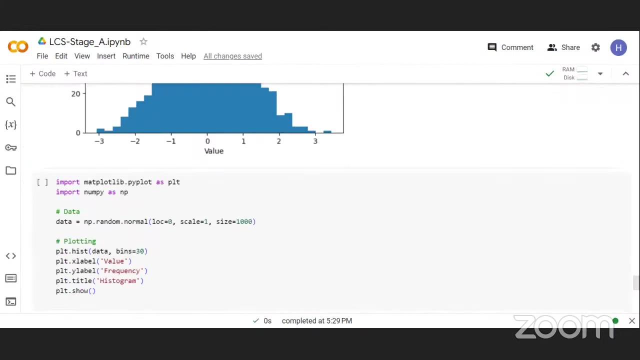 they are not actually all that visually appealing These plots are. they are just the standard plots, So you can just see, to see the data. but the essence of visualization is to have a way to represent your data in an appealing manner. So smartplotlib has provided us with a 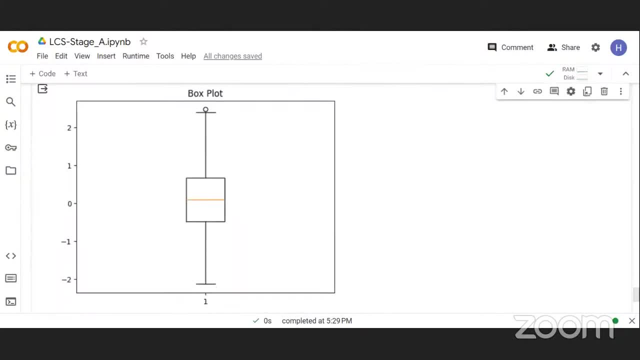 with an array of different features actually that you can use to change the color, change how your plot is being returned and all of those kinds of stuff. So let's say, for example, for this line plot: now, if I try and redo the line plot, 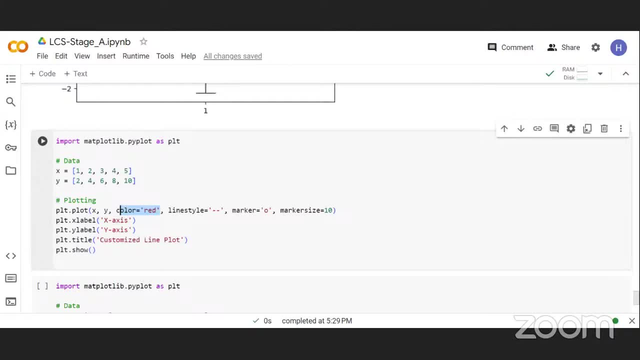 but now I'm saying that for the line plot, let the color be red. And I also want you to the line style. don't let it be just a straight line. It is going to be dotted lines And then I'm going to have a marker. 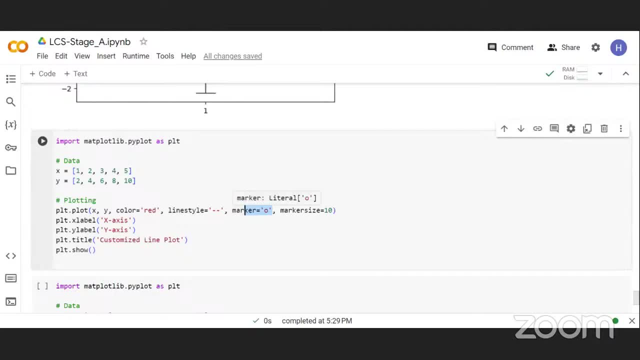 What this marker does is that it gives you. what the marker does is that it tells it's in the line plot. it also shows the points that match. So if I run this code now and you see the value, you can see now that instead of just having a line, 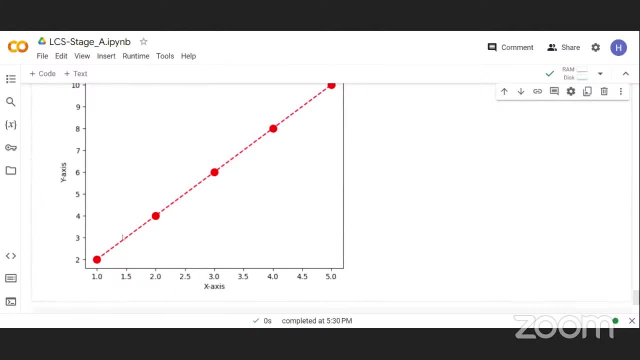 we are now also seeing just as what a scatter plot would have given us. But now we are trying to combine both a scatter plot and a line plot into a way. we are seeing the line And we're also seeing the what. we're also seeing the different values that are attached to this line as a point. 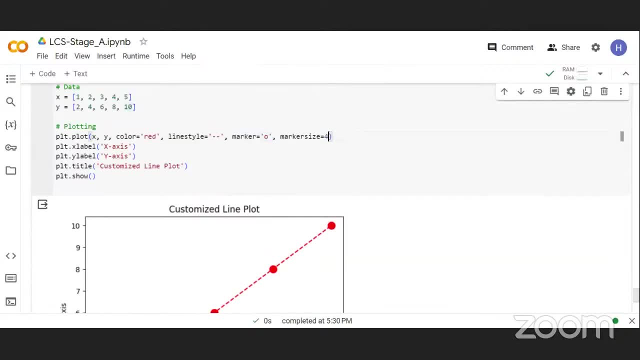 with a marker. So the marker says it's time. So to me this is too big. I can reduce this to four And if I run this code, you see that the marker size would have reduced. And this is the marker. 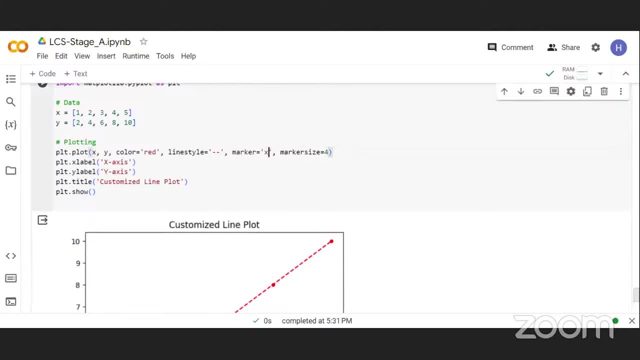 You can also change your marker type. I think you also have the option of X. If you use X instead of O, you can see this is an X. Then I can increase this from four, let's say, to six, And the X would be more evident that. 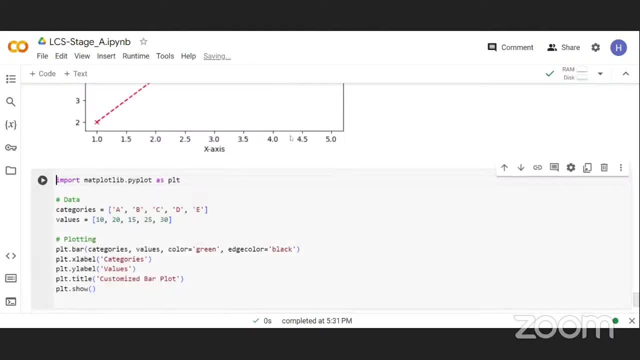 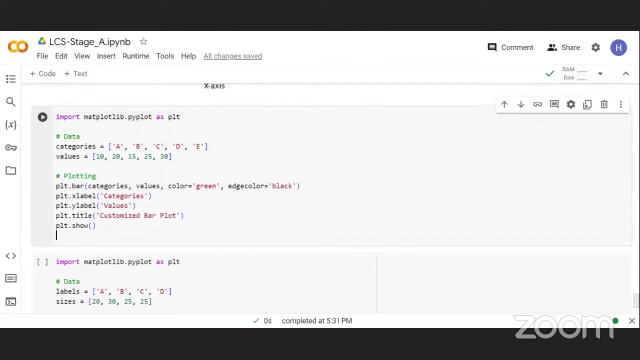 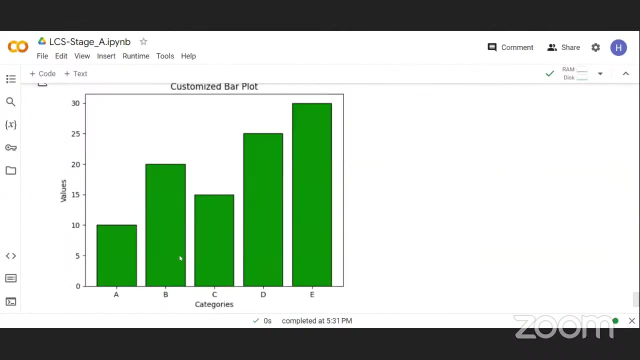 okay, this is the value of these values using X. So that's one way of visualizing. Another way of visualizing is for the bar charts. If I run this code now, you see that the bar charts exactly. So now, instead of it to just be a blue color, that is not appearing. 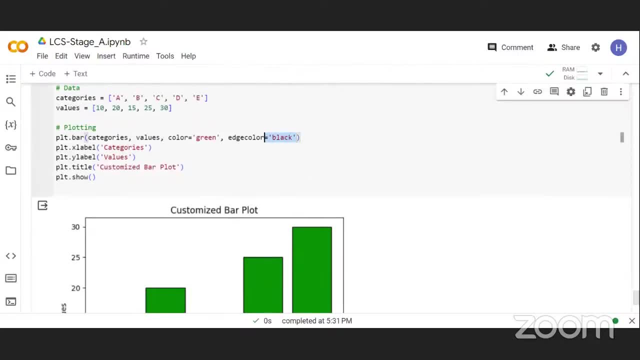 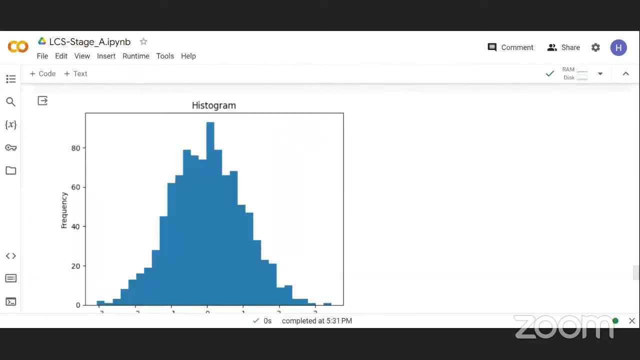 now it's green And we have also specified that the edges should be colored black. So you can see that the black here is more defined than it was in the previous bar charts that we had. You can see the previous bar chart. I don't even think it had any edges. 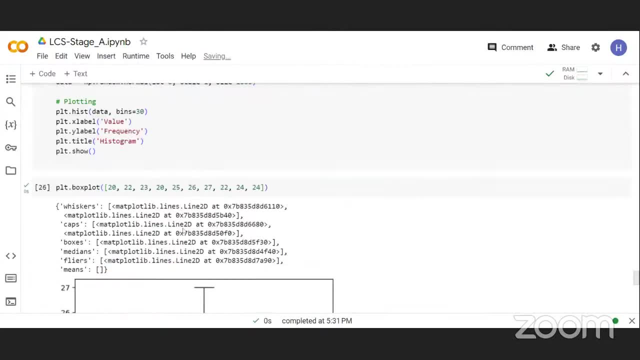 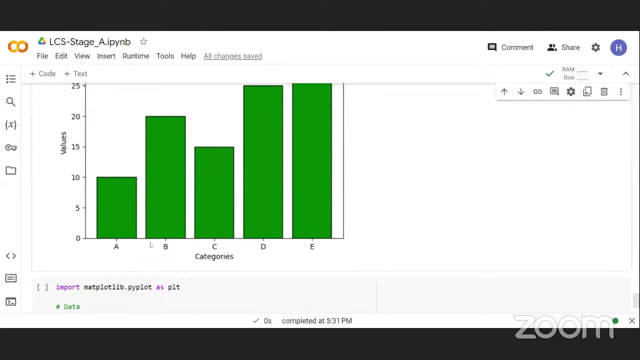 So this was just the color. But now, in this new bar chart, we have tried to define the edges And we have defined the edges in a finer manner. You can see that. okay, these bar charts here. it has this, it has this. 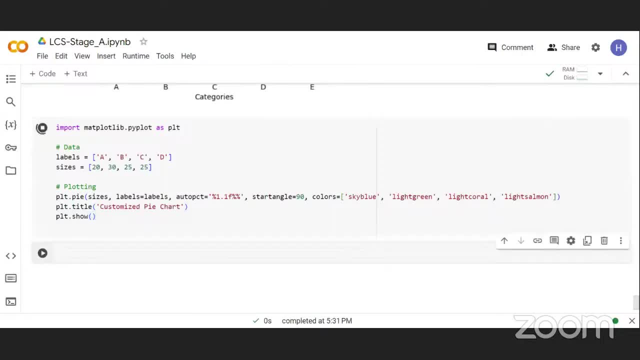 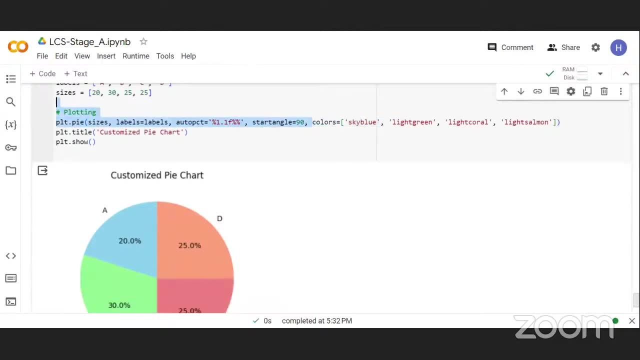 and it has whatever. So for the pie charts, if you try and do this, you can see now the pie charts. we specify that. okay, you should show the value And then you also specify that for each, for each part of the pie chart. 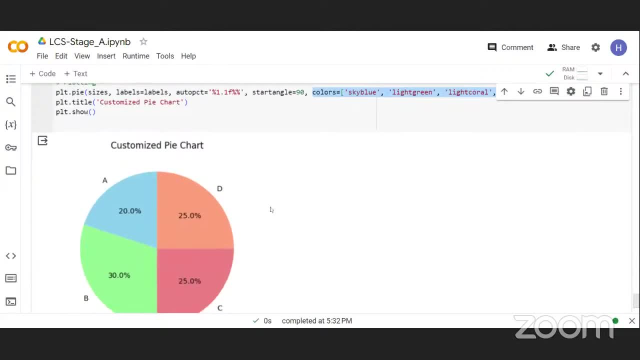 this is the color that corresponds to that part. So yeah, for the color for label A, give it a sky blue color. For label B, give it a light green color. For label C, give it a light coral color. And then for label D, 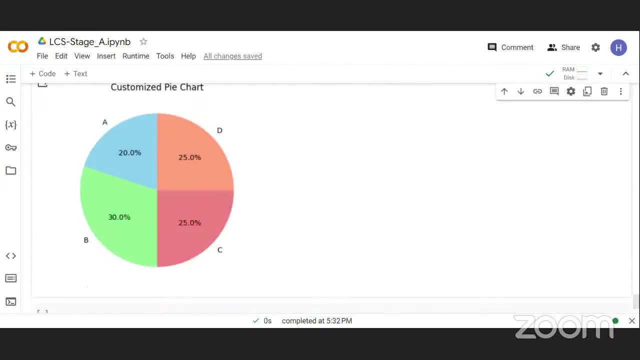 give it a light salmon color. So that is another way that you can like make your charts more visually appealing and work on them in a good manner. So that is basically most of the major things about Matplotlib because, like I said, 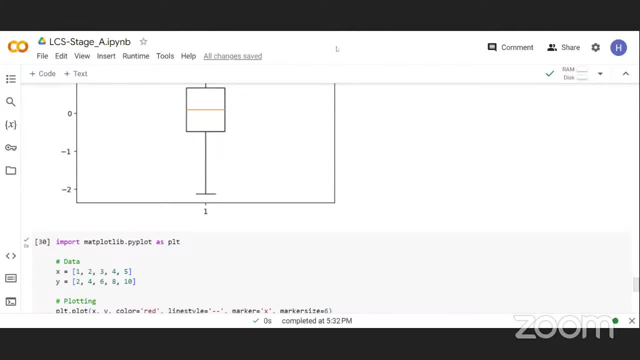 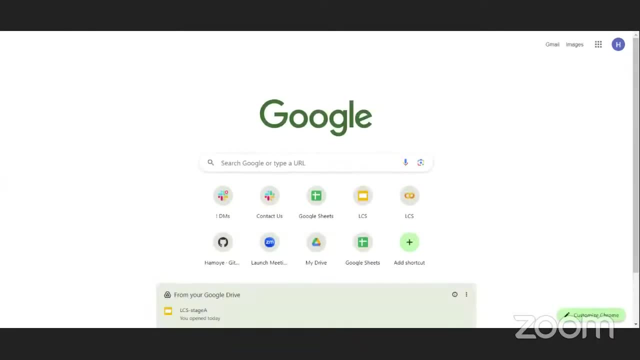 we can't really go through everything in this short time, It's just basically showing you a simple stuff. So, if I share this, my new tab also, just as I said for Pandas, for W3Schools again also serve as one of the best places. 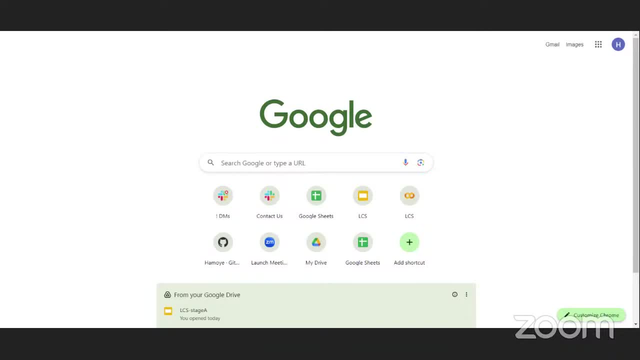 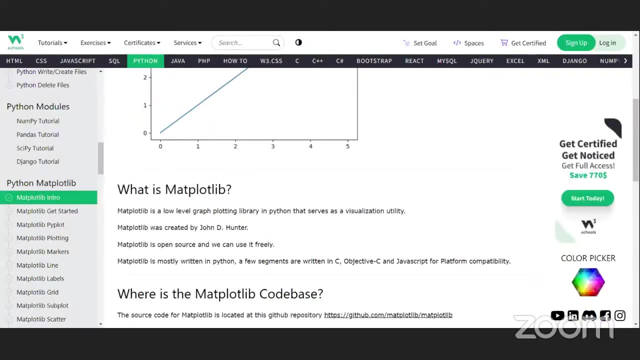 So, rather than Pandas, just put Matplotlib. So if you go to W3Schools for Matplotlib, they have a lot of what? a lot of different tutorials for how you can use it. What's the Matplotlib getting started? 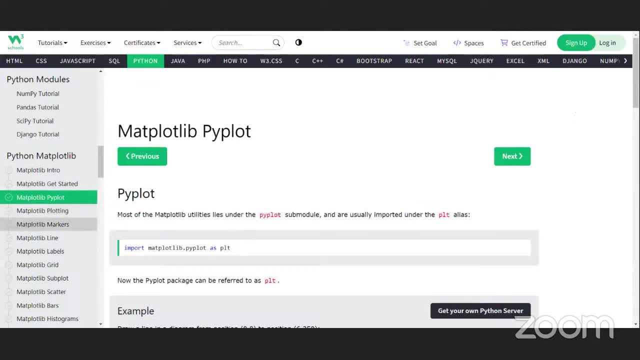 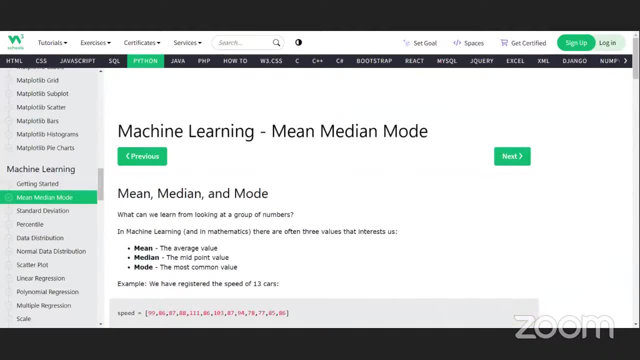 you install it and then what's PyPlot? how you can start plotting with different things. They have a lot of grids. how you can use this, the mean and median mode, even in W3Schools, to try and use NumPy. 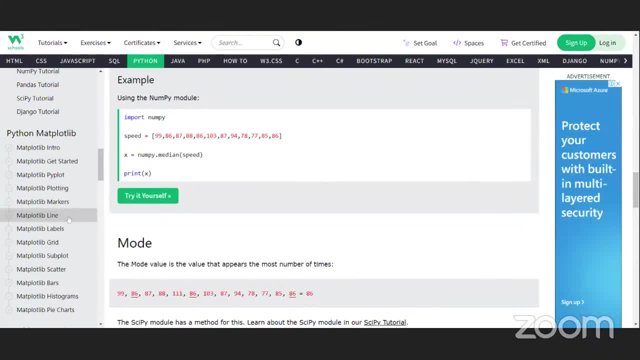 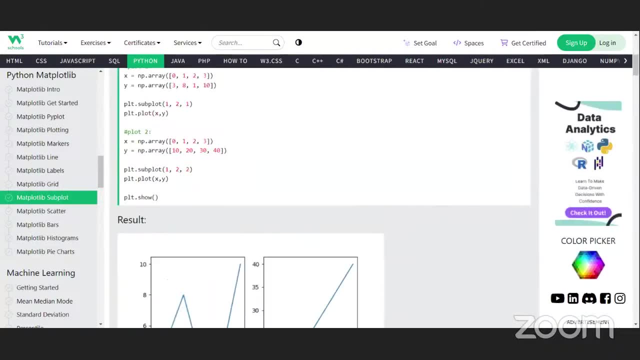 and then try and visualize all of your data. So part charts, lines, labels, how to use subplots: Subplots is something that you should learn how to use a lot, because with subplots you can see you can create more than one visualization in the same figure. 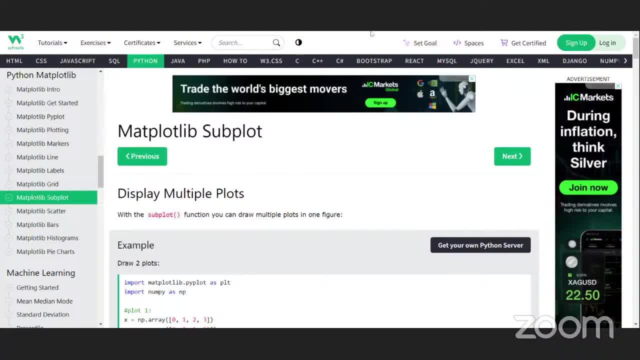 And these are a lot of different things that over time, in your next live coding session- because we are still going to expand more on this as the guy for the data storytelling track moves to the abstract- you'll see a lot of different tools that you can use for visualization. 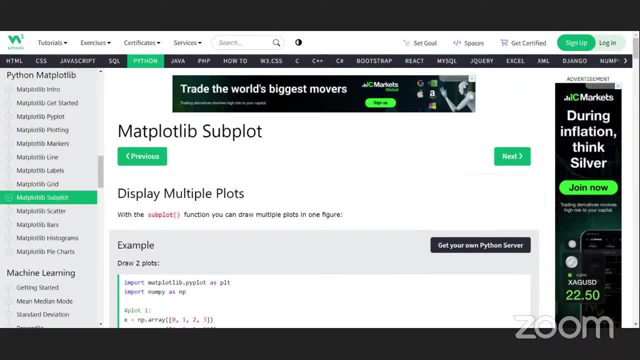 Even, rather than away from Python. you'll be introduced to no code tools where you just provide your data set and then you drag and drop the kind of visualization you want. And you'll also be introduced to more, more technical Python commands. 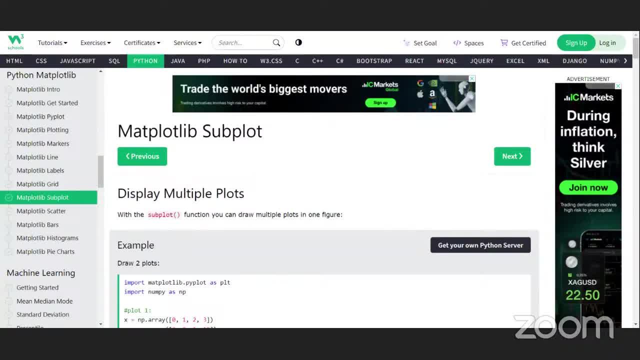 and Python functions that you can use to create more visualizations And also even for the machine learning guys. also, you'll see the aspect of EDA and how you can use the inferences that you use from your EDA to inform the kind of machine learning model that you'll be training on your data sets. 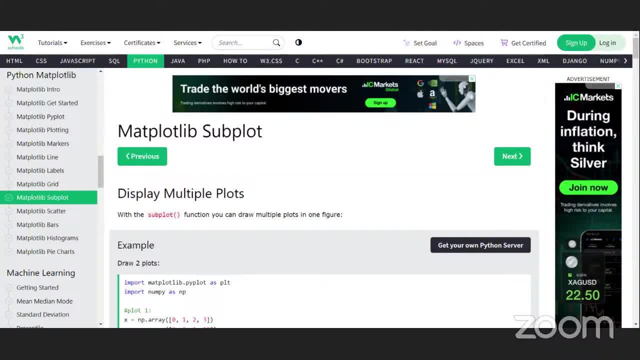 or whatever, or whatever it is that you are going to be doing. Yes, since today is the last live coding session. since today is the last live coding session. since today is the last live coding session, the notebook and the collab. 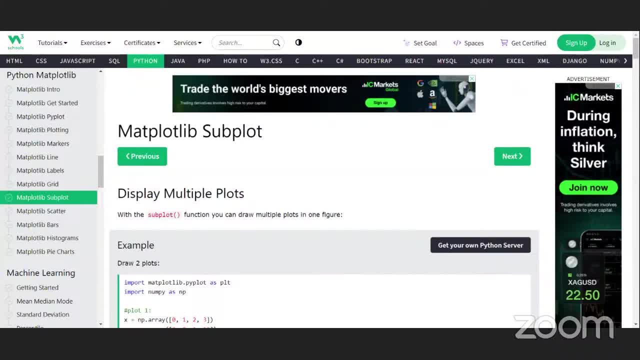 the notebook and the slide will be shared immediately after the session. And then I saw something about Seaborn. Yes, for guys that are going to the Python storytelling, you'll use Seaborn a lot, And in the next live coding session that you have, 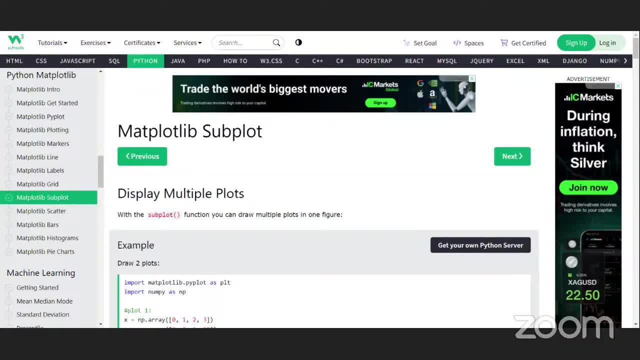 you'll be introduced to Seaborn and how you can use all of this to make most of this blood. Seaborn is something that was built off on Matplotlib and they work hand in hand, So there were some tools and features that data scientists wanted. 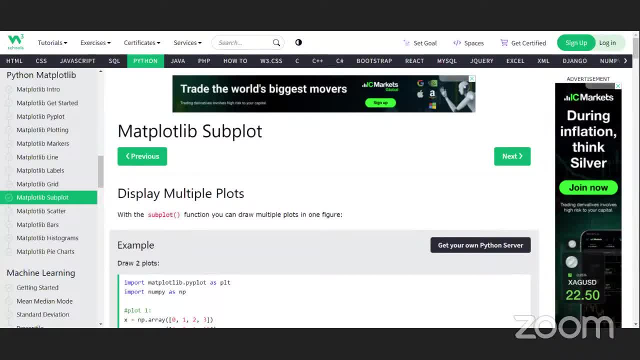 when visualizing data that were not provided in Matplotlib. And when Matplotlib was created it might have taken a lot of coding variants to create those in Matplotlib. So Seaborn is a module that was born from Matplotlib to try and bring all of these visualizations. 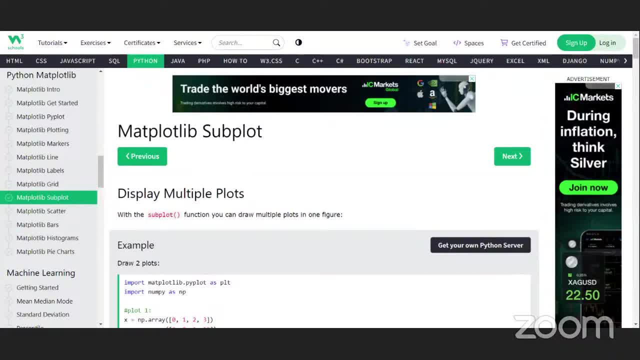 and add more customizations, more colors and a lot of different things that one can use to navigate and do a data storytelling. So today we have come to the end of the live coding session And I just want to open doors for maybe questions and stuff like that. 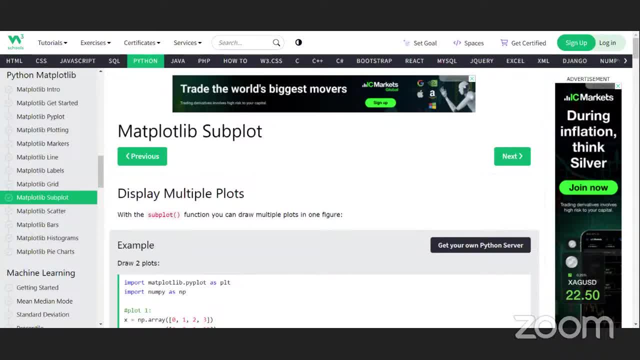 before we end the session, because it's the last live coding session- then, From the next stage, everyone will have been shared into their respective groups, where, in your respective groups, as I've stated, you start going deeper into whatever track or specialization you have chosen. 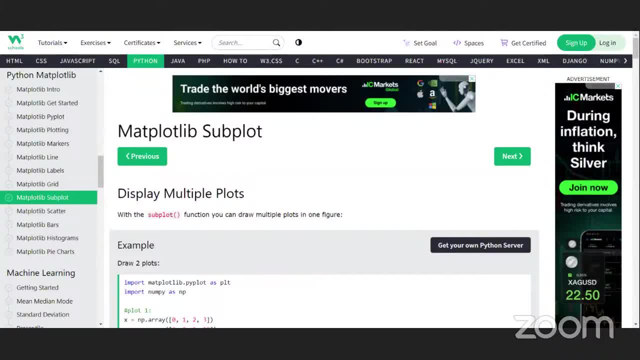 So, any question, My name is Adenyo. My name is Adenyo. Adenyo Angulabi is my name, And this is going to be my last session with most of you, But from the next, live coding session, 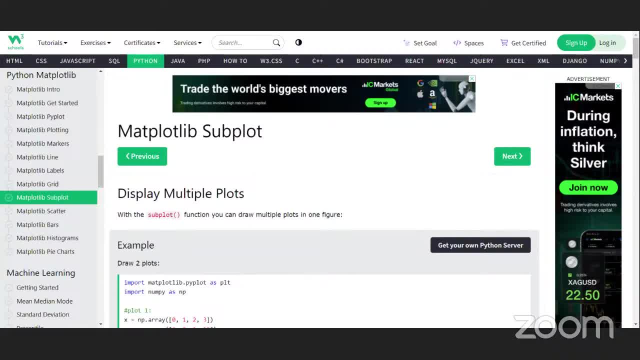 I'll be focusing more on the DevOps guys And your facilitators, for the next live coding session will be introduced to you very shortly, And you also have a wonderful time of learning with them also. So Hakeem has his hand raised up. 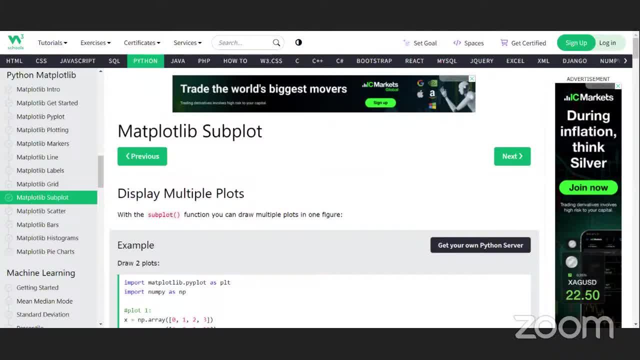 Hakeem your question. Okay, I think that was a mistake from his side. That was a mistake from his end, Okay. So with that, I think we have come to the end of the live coding session. And what time is this stage? 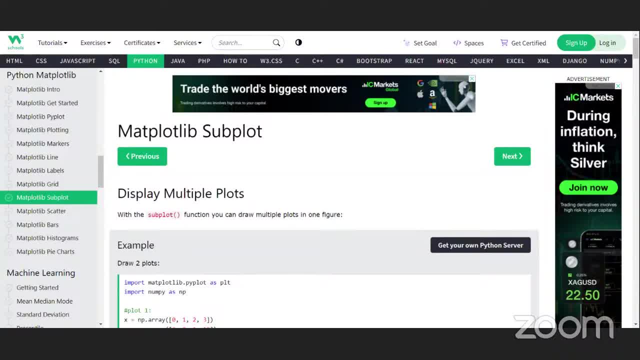 A quiz closing. So the quizzes close at 12 am. So the last time you have tomorrow to submit, to make any submission, is 11.59.. After 11.59, everything is going to get reset And then. 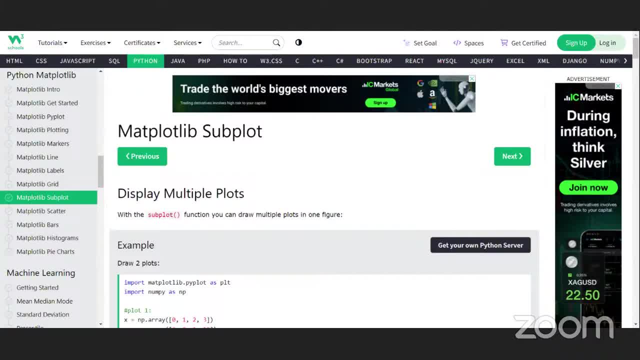 if you have not done any quiz, you cannot take it anymore. How much of coding do we have to do? Not much of coding. I think the quiz is a total of 20 questions And then just about, I think, less than 10 questions. 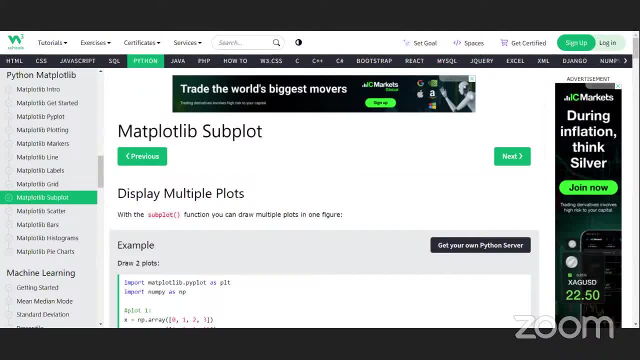 are related to the data set. Some of the questions are related to concept and text materials. that text materials, that are we getting text materials in the text materials in the in the course, And then the meaning is based on the data sets. 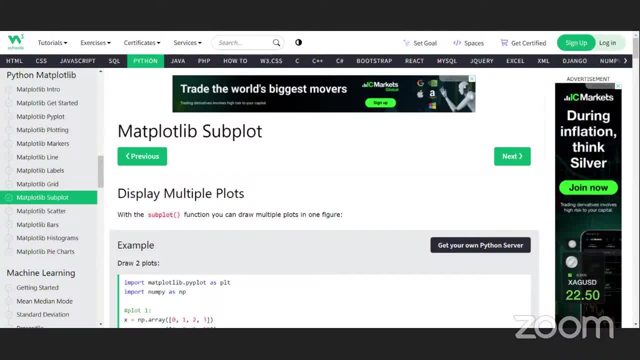 So the stage ALCS resource, it will be on Slack, which is going to be on Slack. We'll post it on Slack on the announcement channel for everyone to be able to have access to it. And then someone does ask if I can expand it on how to use group by. 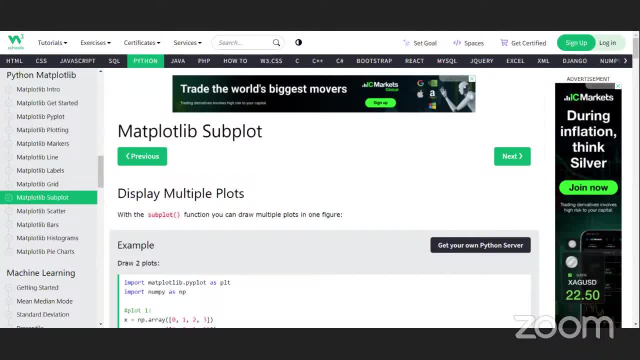 So I said this- I think that was two coding sessions ago. Group by is a method for trying to group your data sets by by a category, that a category that is easily available. Let me see if I can. just let me see if I can try and load in a sample data set. 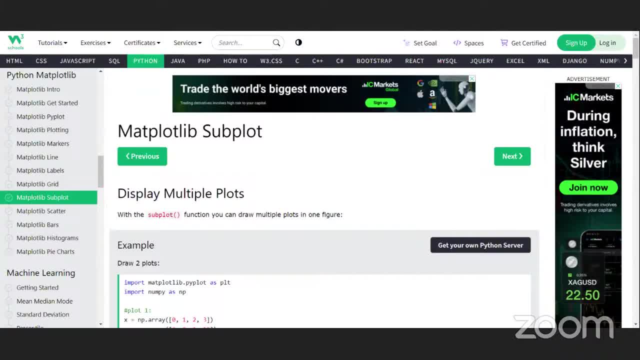 Okay, we have sample data sets here. Okay, Yeah, this, this could. this can also work. So when you open Collab, Collab give you some sample data sets. So let me just say: df is equals to: 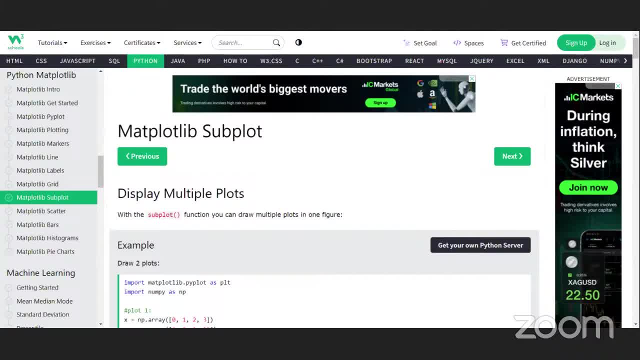 I don't think I imported pandas. pandas previously imports pandas as pd, So df is equal to pd dot. read underscore csv. So let me pick up California housing tests. Let me copy these parts and then let me paste it here: 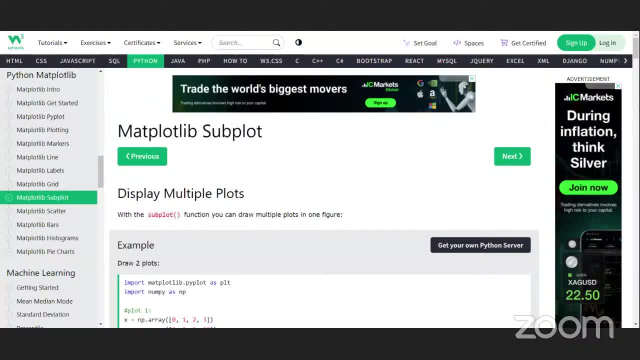 So this is our df. So if I do df dot ed, so with our df dot ed these are the different values that we have in the California. So we have the median age, the total bedrooms population, also median income. 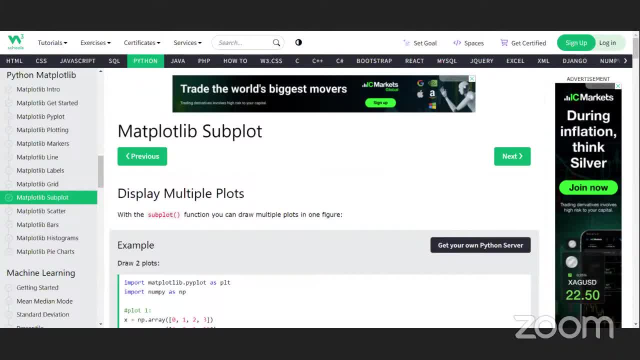 blah, blah, blah and stuff like that. Let me try and see all of the different. I think these are the different columns that we have, but this column though, if I do df dot info. let me see households Sometimes. 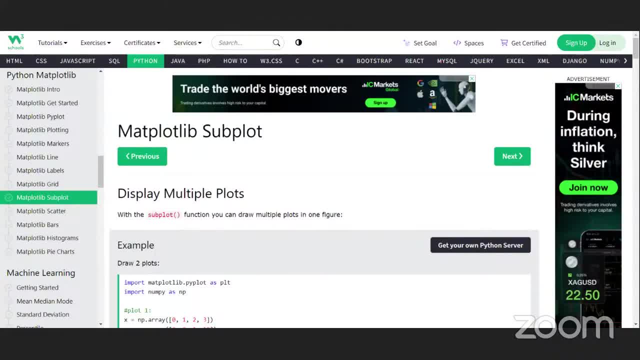 I'm trying to look for a category that I can use. All of these are numbers. I'm trying to look for a category that I can use to, that I can use to showcase. i can use to showcase, um, the goodbye function, let me see. let me see the total bedrooms. 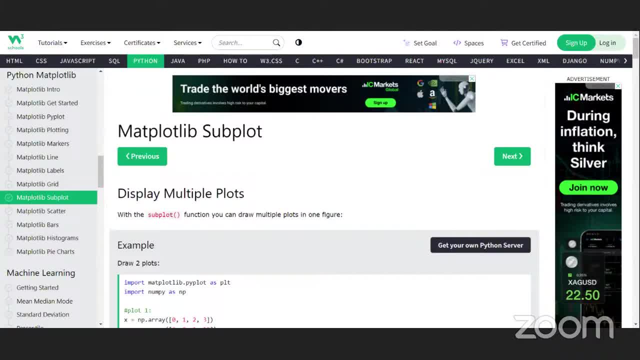 df total underscore bedrooms distribution. so this cannot be used because the values are a lot. the values are a lot, um, okay, let me just try and upload one for my, let me try and upload one for my game. so now let me even this data, this datacsv. 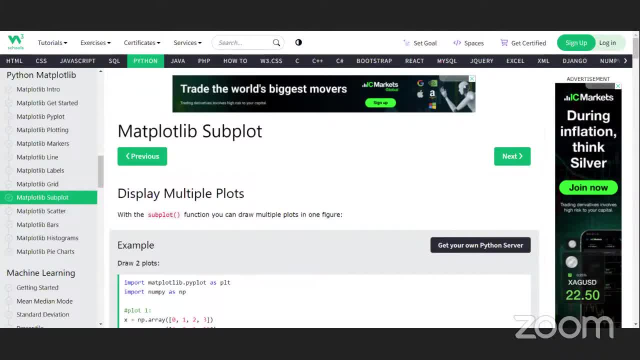 so let me do dfed now. so here we have exactly. so this is the data set to use last time. so let's say for this: um, you know it's possible to have people that have the same education or people that have the same gender. so let me do something here, let me do group by. so when you use group by, you need to um. 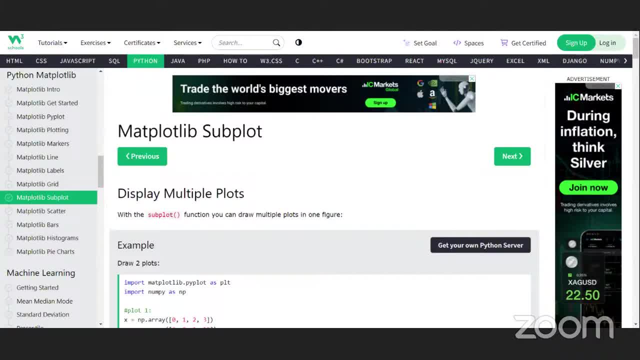 you need to specify the column that you want to group the value by. so in this data set now i want to group it by the gender. so i'm going to say gender and then when you do a good bye, you can't just see the value of what. 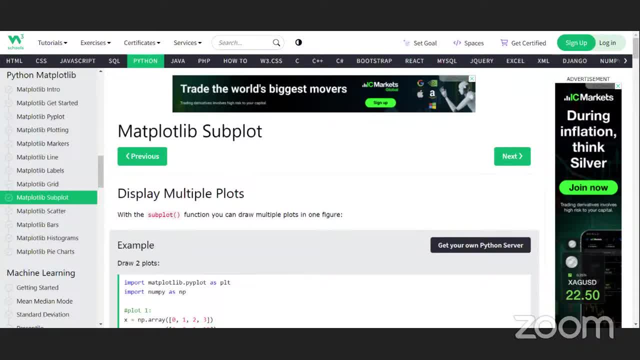 you did. you have to like perform and up you have to. you have to like perform reaction before you can see a value, because the group by object is like: it gives you its first matrix. so it's a good body. so let me say i do something now: dot sum, for example. when i do this now you 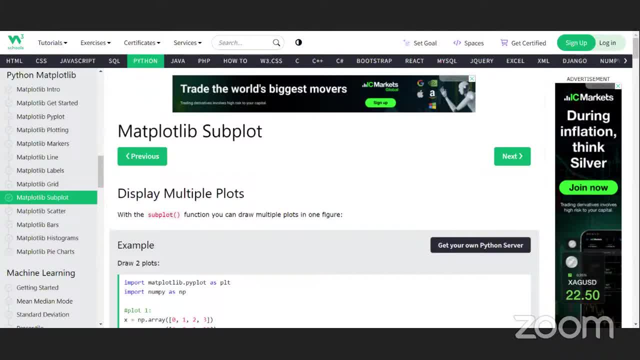 will now see that the result is going to be just the two different unique things that are existing in what you are grouping by. so i'm grouping by what? by gender, so when i'm doing so, so every value in that data set that belongs to the female gender. it will sum it up, but because this is a 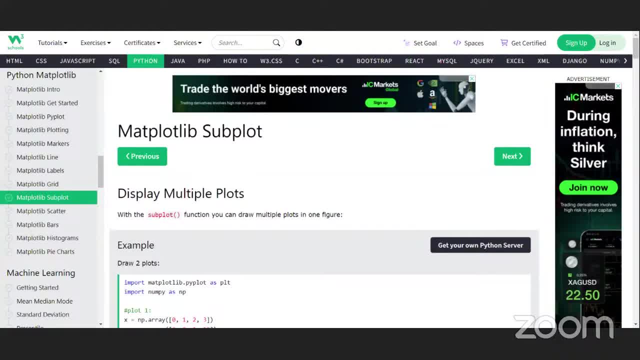 text and not a value. so that's why it's just adding all the things together and then these are the names of all the guys and then the female total age. so by some of the age of every female in the world in the data set is up to 256. the city of every female disease, the total salary of females. 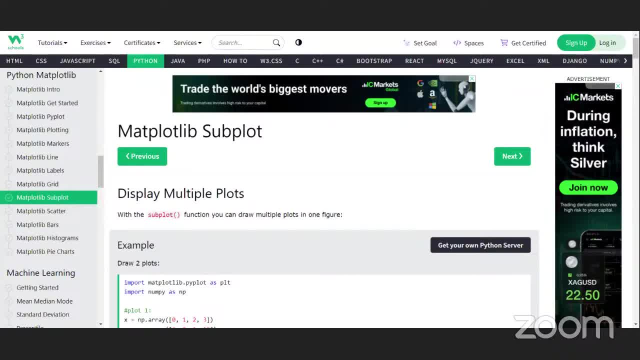 is this, and so these are. you do goodbye, so when you do a goodbye you also need to perform an option. so what goodbye does is, when you go by a particular column, it checks each of the unique value in that column and then extracts every rule where that particular column is equal to the coin. 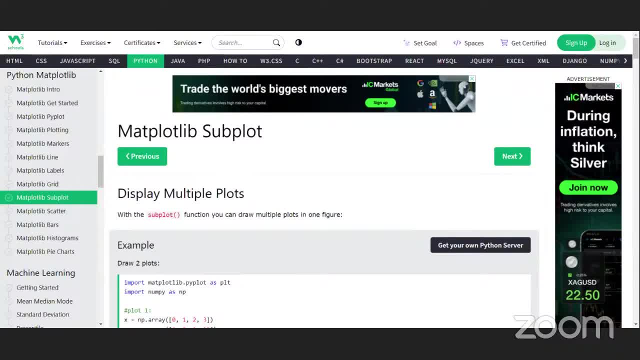 so if i do something like this, now, when you do a google, there's something called get groups, if i remember, if i'm correct, get groups, and if you do this, okay, there's no guest groups. i think it should be groups, exactly. so when you do god groups, you can see. this is telling you that after i perform this. 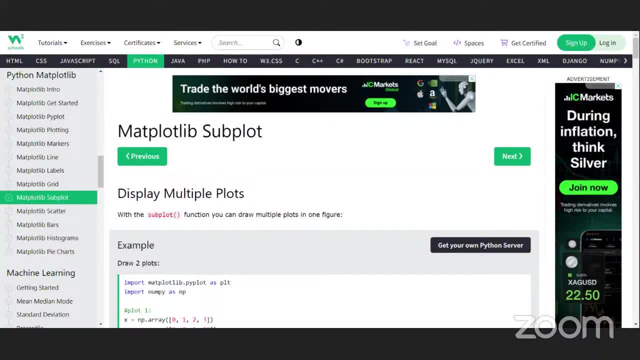 group on the data set. we have what females and what and news. so every female, so the the who that is of you say: okay, rather than looking about the gender, now let me book by the city and do the same thing. you see that we have different cities, so we have boston. 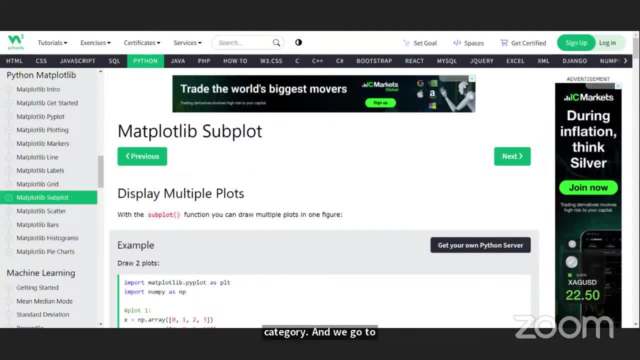 in this data set. we have people that also come chicago, other people from los angeles, the other people from military state. you see that we don't have at least. so all of these cible. we are at least to get the equality we are getting from america in the data set. so that means that we got 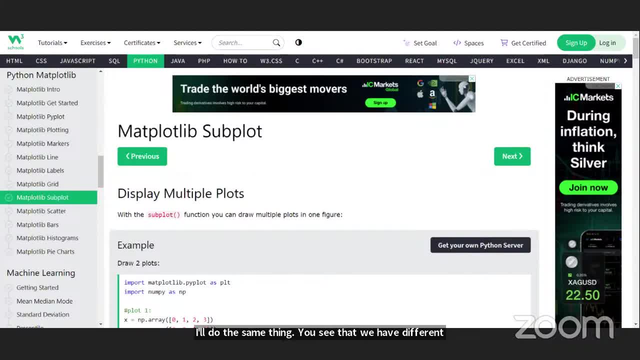 equality, likezo here. so that means we now so the gender of this group, where we are also good. so but 竿 people from new york, from san francisco. so the row of row 5 and 11, those are the people that belong to boston. the people in row 2, 8, 14 are from chicago, and then people in 1- 17, 13 are in. 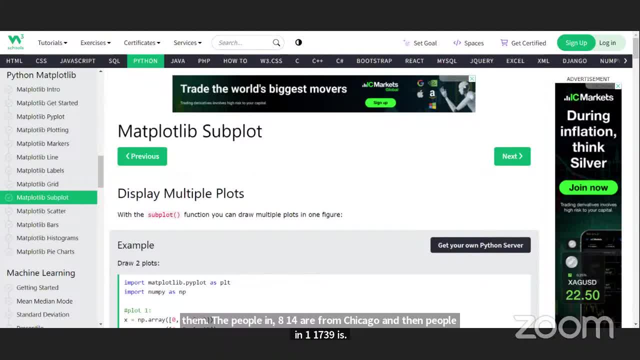 los angeles. so what? that's what group by does? it allows you to take a particular column where it's their categorical variables. so you cannot use. you cannot try to do a group by with the age column, for example. it does not make sense because there is lesser possibility for different people. 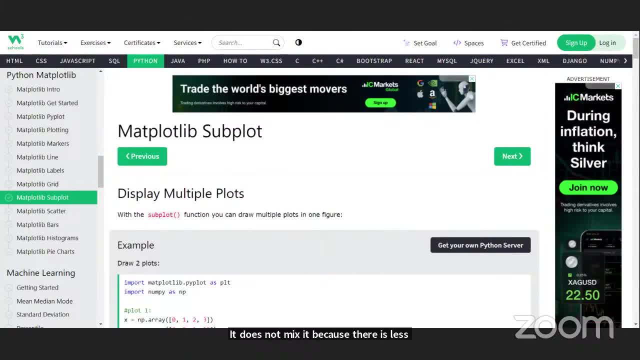 to have the same age range than the possibility of people to come from the same place. so most times when you want to do a group by, you do a group by, um, you do a group by. oh, you are not seeing my collab screen, sorry, somebody should have. somebody should have tried. 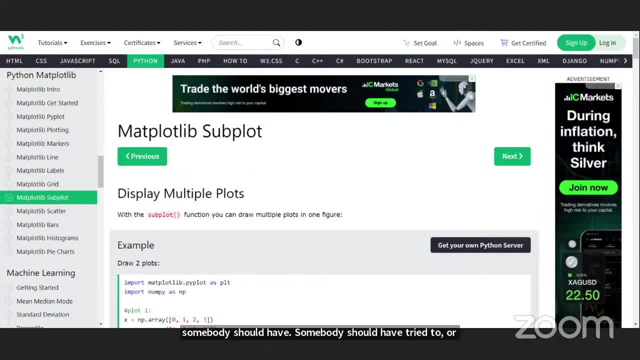 to um unmute in in camps like this, when you, when it's probably something about my screen and stuff, you just try to like unmute and tell me sorry for that. i i thought i was sharing my. i thought i was sharing my window, not my um club. so let me share this tab. 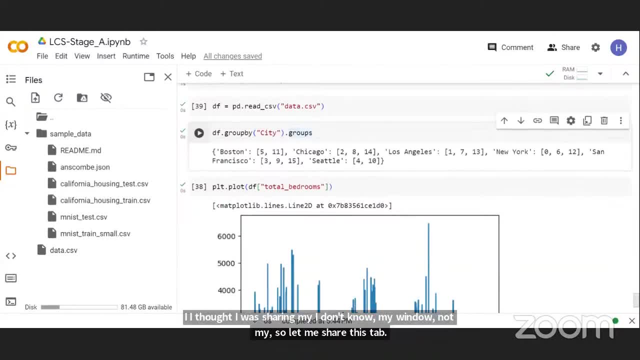 so you can confirm now that you can. oh, our green has locked ability for you guys to unmute. oh, i see. apologies for that. next time i'll be sharing my window rather than my screen, so we won't be having this issue. but yes, what i did was i first read this data setting. 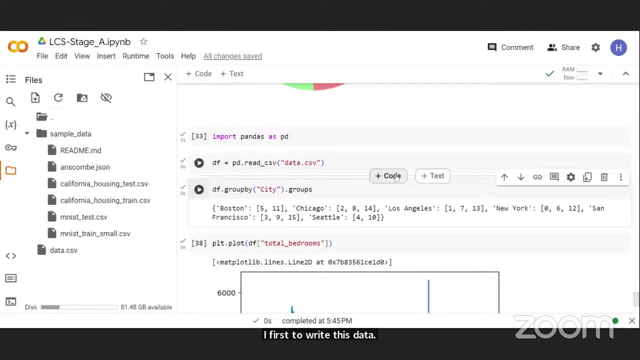 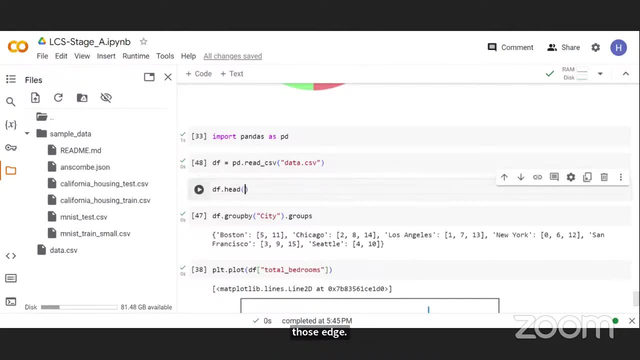 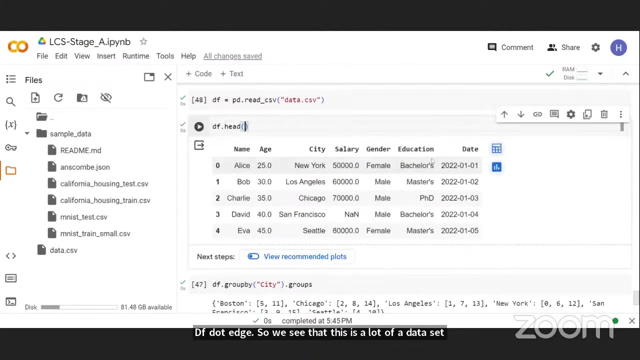 so i read this data setting and then, if i do, like a dfed, dfed. so you see that this is a lot of um, a data set that contains the name of people, the age of people, their city, salary, gender, education and what have you. so, um, when you 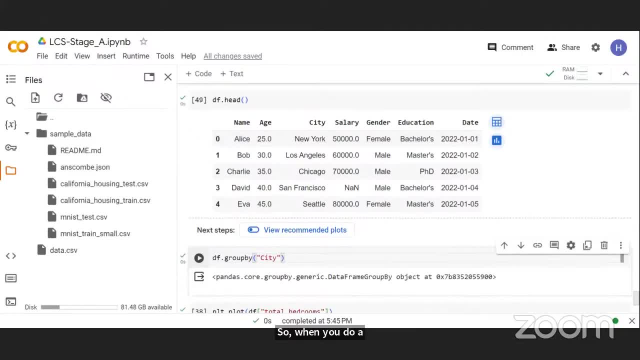 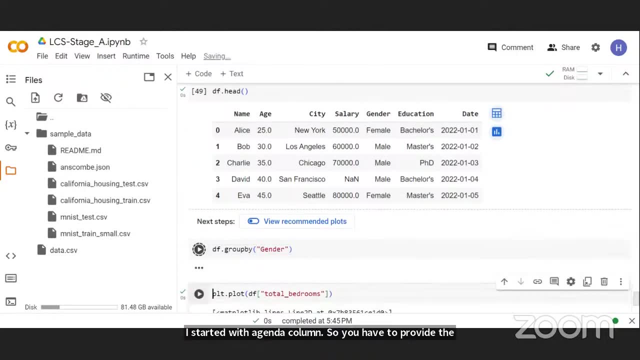 do a goodbye. i was showing that if you just do this to do a goodbye, i started with the gender column, so you have to provide the name of the column that you want to go the data set by. so yeah, i'm providing the gender column as um. 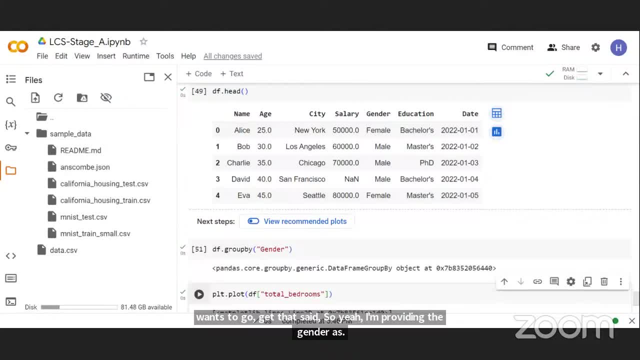 i'm providing the hope. you guys can see my screen now. if you can see my screen, i can just like send emojis or something. okay, yes, you can. you can see my screen. yeah, thank you. so let me continue. okay, so, let me continue. so, as i said, when you perform a group by function, 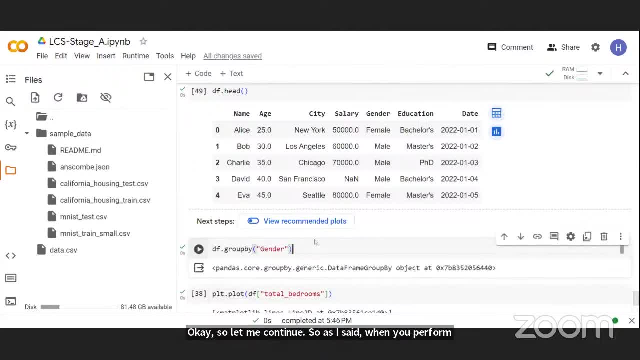 what is returned to you by pandas is a generic object that you cannot access like that. so if i google by general now say: let me try and access the age or something, um, you see, even trying to access the age is going to be a generic object before you can see, um, the values of what your group, by, is going to give you. you need to perform. 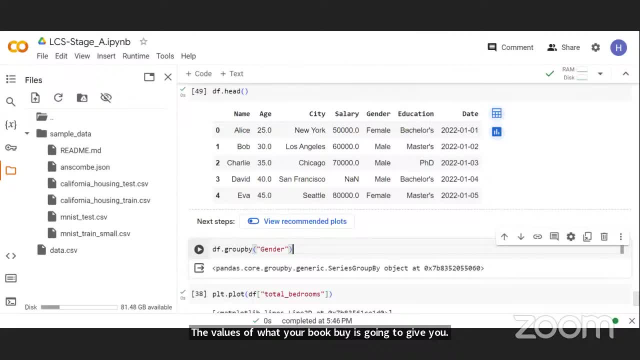 an aggregation function, so aggregation function is like function that combines different values together. the major aggregation functions that we follow for entrepreneurship partners, which are the most convenient version of the gdc- like you need to do gdc to find up to size- thoseека and internet: 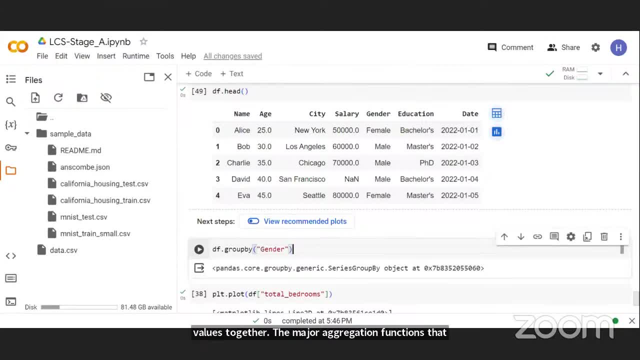 you also need to perform integration functions, so aggregation function is like a function that combines different values together. the major aggregation functions that provided are the main function and the sum function. we also have something called the math function. we also have the main function, but the major ones that we use are the main function. 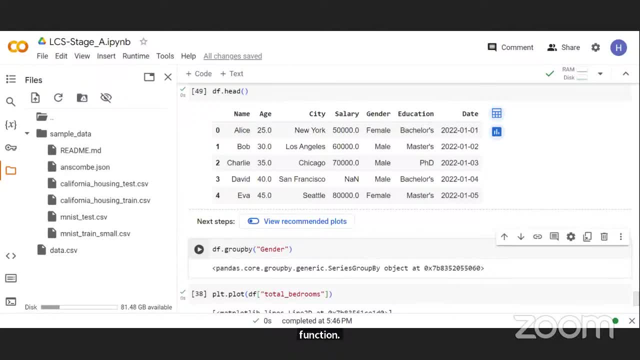 and the sum function because the idea is that when you are grouping by a particular column, you want to see the set of values that belong to that column or something. so in this column, for example, i have grouped by the ginger, so i want to see- okay, let me try and see that- what is the? 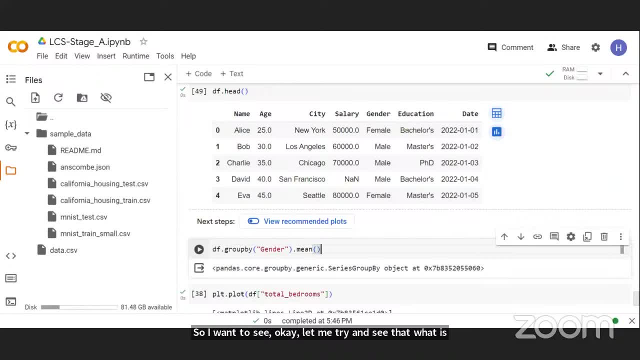 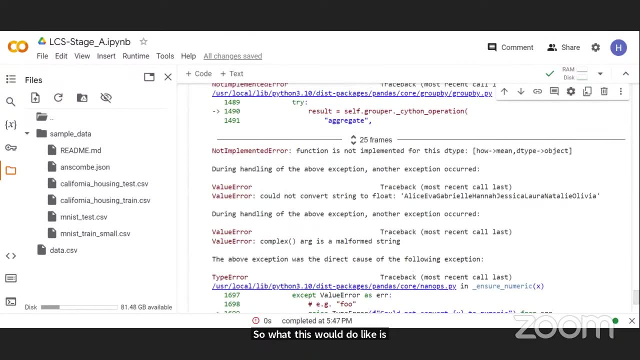 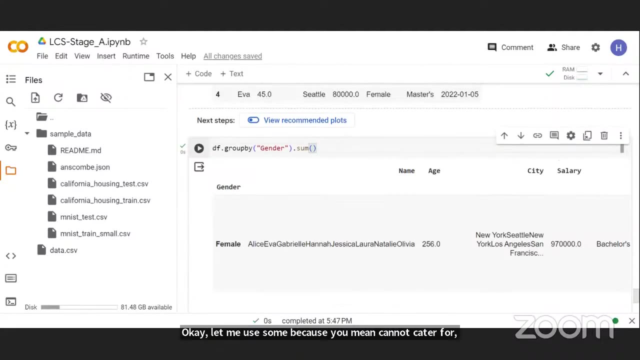 minimum value of the salary of people that are in different genders. so what this will do now is it will go to the gender selects. okay, let me use some, because you mean: cannot cater for um texts, some can cater for text. so what is doing? i can see in this gender we have just two different. 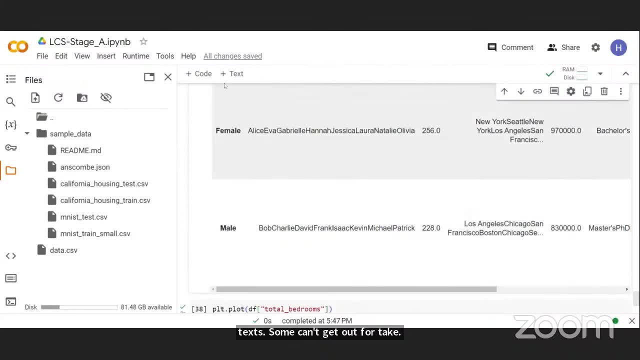 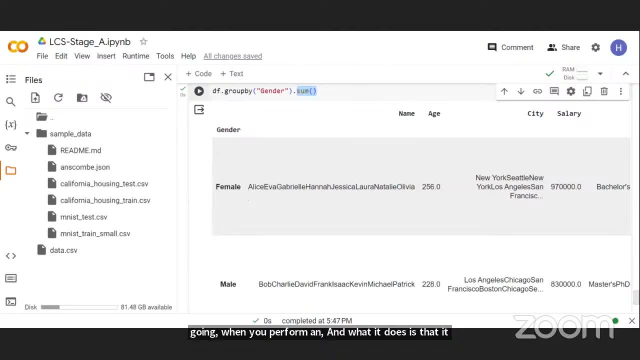 through the data set and for each of them it selects the rules that belong to a particular group, a unique group, and then perform the aggregation function on them. so for, basically, for the female group, these are the summation of the names of every female in the data set. 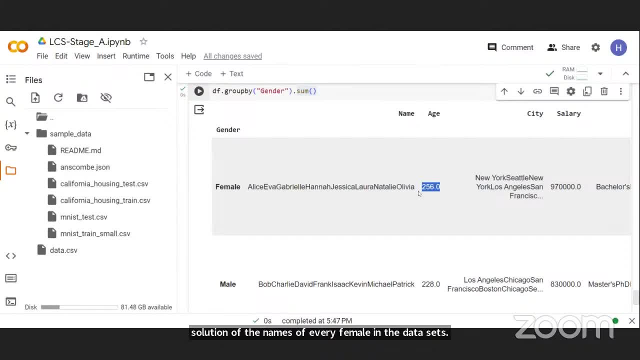 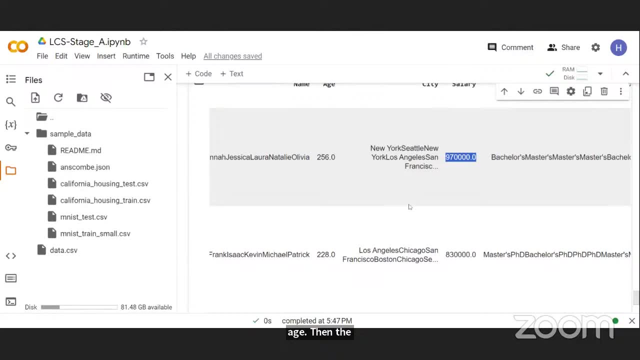 the total age of every female data set is 256 years of age, then the summation of the different cities that they come from and then the sum of their salary is 170 000.. it's the same thing for me too. it sums up all of the names. 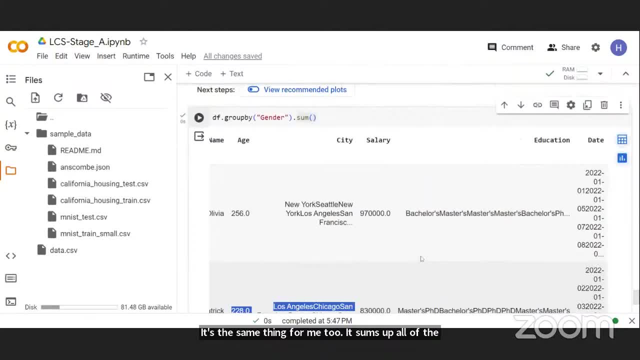 sums up um, the age of all of the men, and something like that. so the way it works is that when you do it, so there's this function called those groups, or it's not a function. i think it's a. it's a method, because you cannot call it. so when you call this method, what this does is that. 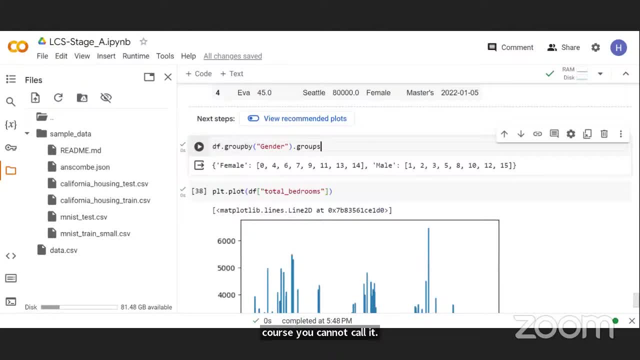 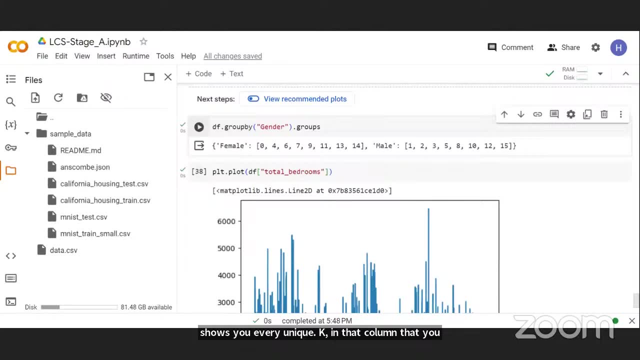 it shows you every unique category in that column that you specified and each of the road that corresponds to that category. so, basically, in this data set now for the female category: um, zero, zero, four or six, up to 14. these are the rules that when you check the agenda they are. 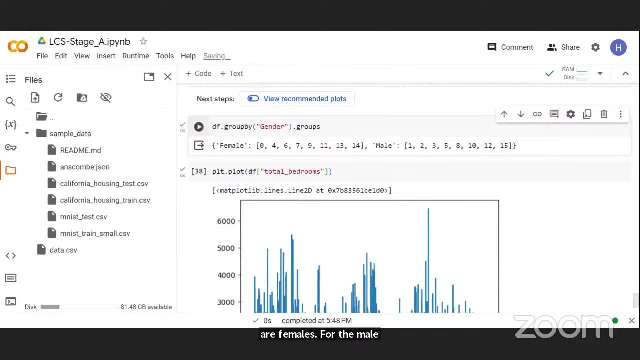 females for the male category: one or two or three or five, eight, ten up to fifteen. these are the rules that when you check the agenda they are in the new category. so this is how this is what group by does. so let me say, i change this now from gender, let me change this to city. 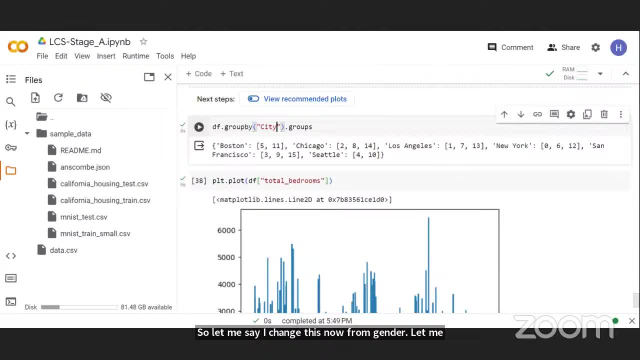 and if i change this to city, you can see now, now we have a lot more city. so, um, instead of those two, we have boston, people from boston. the only rules where, if you check their city, they are from boston is what will? 5 and 11.. for chicago, it is row 2, 8, 14.. los angeles is 1, 7 and 13.. in new york you 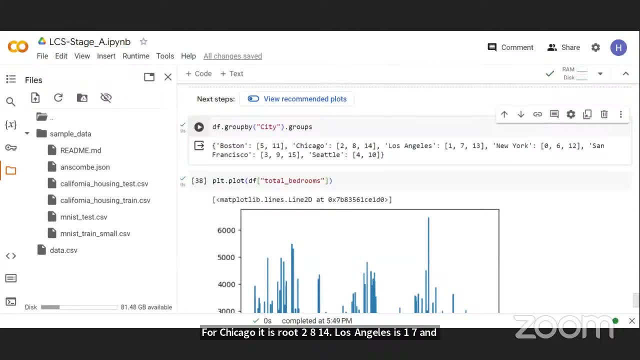 have 0 or 6 hours and the like. so when you use a goodbye function, that's what it does. you use that color to check the different unique values that are in that column. after you check the different unique values that are in that column, you can then 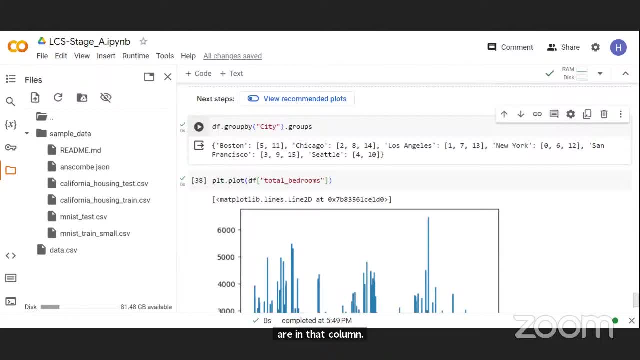 try to like. um, you can then try to like show each of these values. so if i let's say, for example, i know that, okay, boston is actually a group here. if i copy boston, i'll now do this, say get group, and i'll put boston here if i want this, this will not give me all of the rules that belong to what. 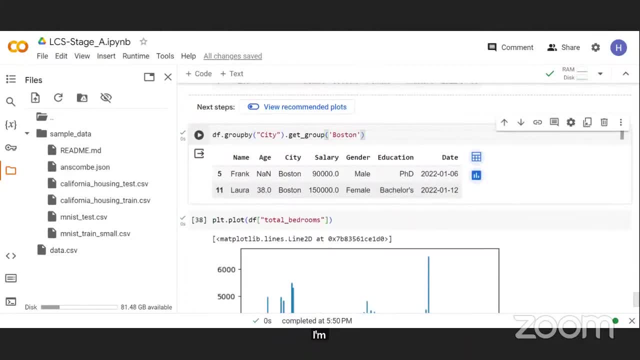 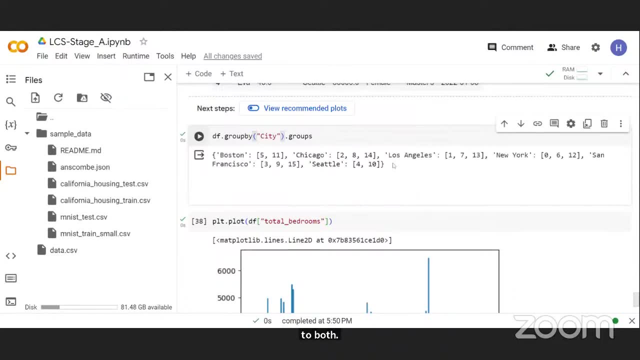 that belong to boston. so if i just um take this away and try to get another one, i will put boston here, and then i'll put boston here, and then i'll put boston here, and then i'll put boston here. another group, let me say los angeles. 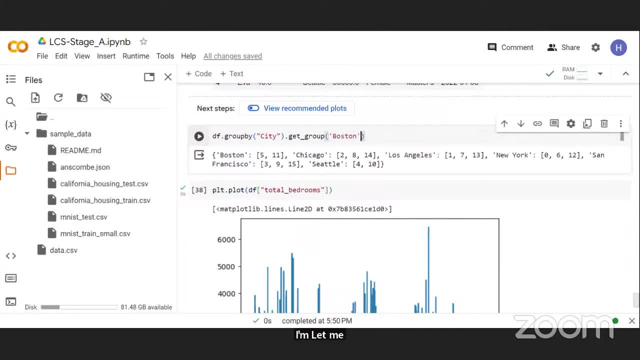 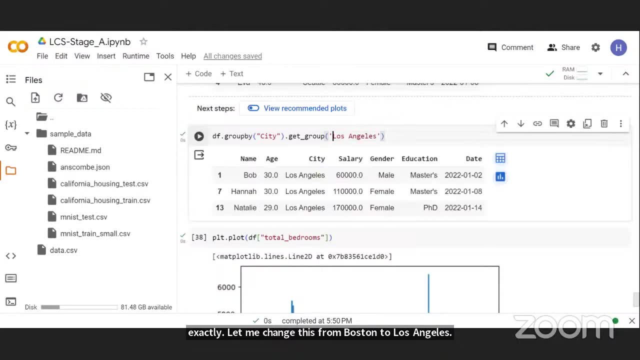 let me say los angeles, and then let me use control y, exactly, let me change this from boston to los angeles. what this will do is it will go to the game. so, after i perform a goodbye, the only way you can see the values that belong to a particular group without performing an 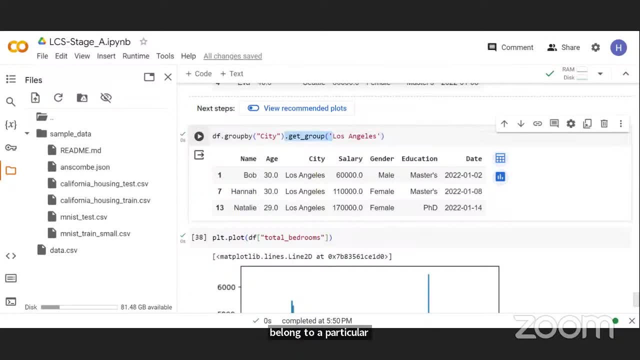 abbreviation function is: if you use this, get group function. but most times when we do a goodbye, we just want to do like a, we want to do like a, a summation to see, okay, in this particular group, what is their mean value. so something like this- now i can do- counts. 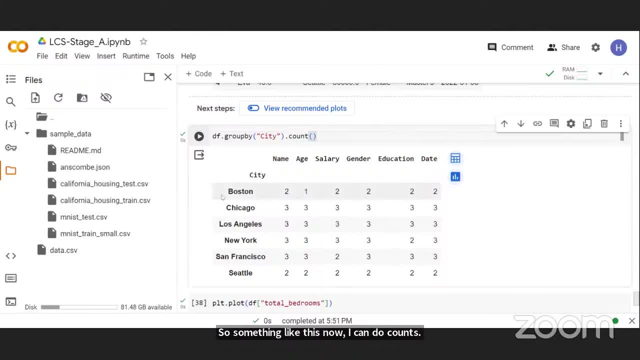 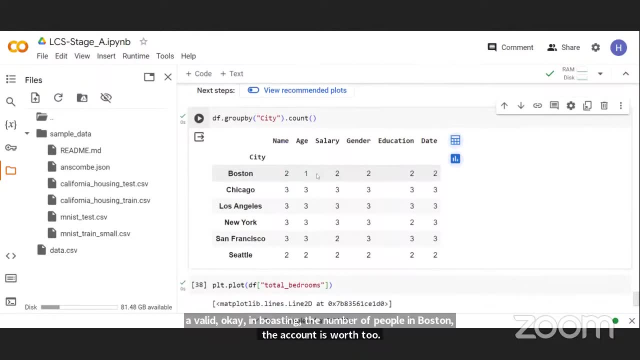 so you can see that with this. now this is returning the value. okay, in boston, the number of people in boston, the account is what: two, the age is one, salary is two, so that means somebody in boston. now, the age was not present in this data set for chicago. 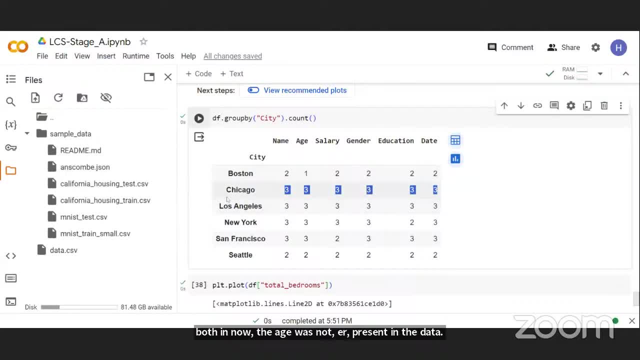 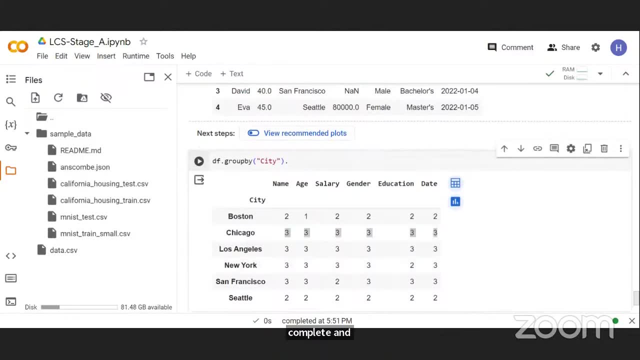 we have what? three people? three people, so that means everybody that belongs to chicago, every of them was complete and stuff like that. so let me say, for example: now i want to do, i want to check, i want to use a bar chart to know the mean salary of different people that come from a particular 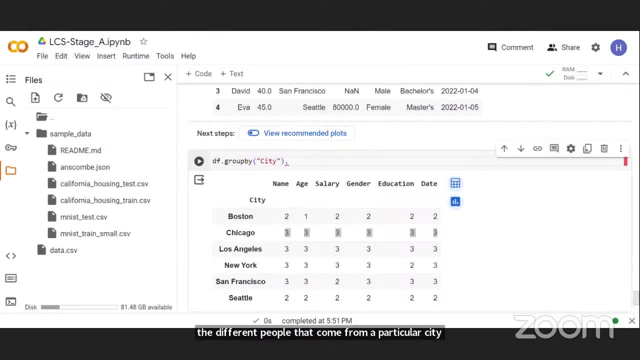 city. so after grouping by a city, now i will get the mean or no. after grouping by the city, now i can get the mean. okay, but before i get the name it does get the salary column, since i know that i'm trying to get a mean and the main cannot work with. 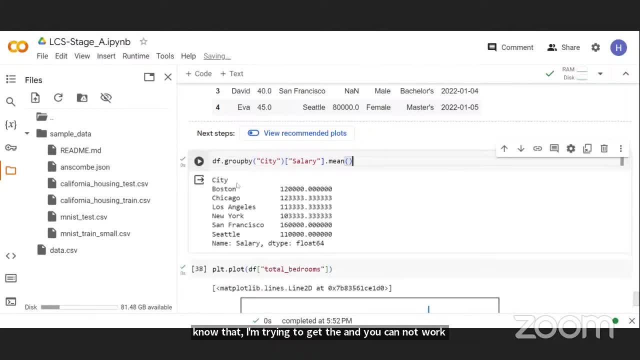 this. so if i do this so you can see for each city: in boston, their mean salary was what? 120 000. in chicago, their mean salary was 123. but rather than seeing this as a value fund, that's also performance, with something called dot plots. 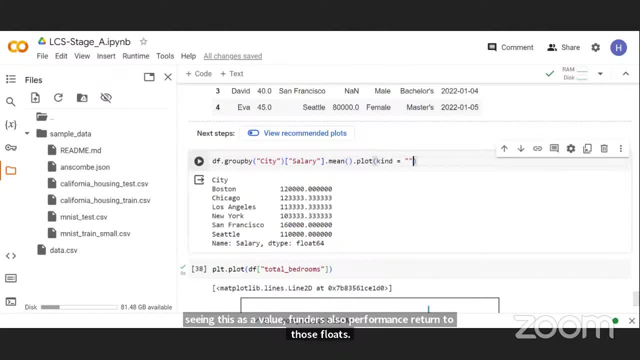 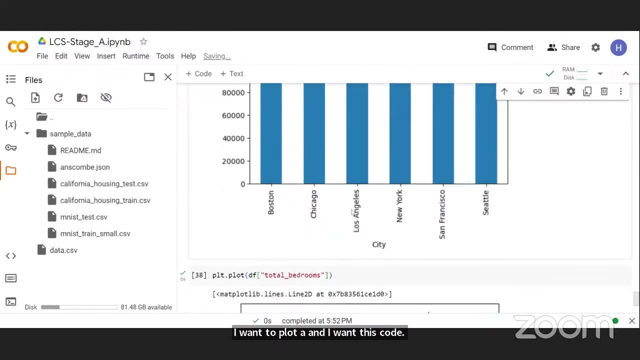 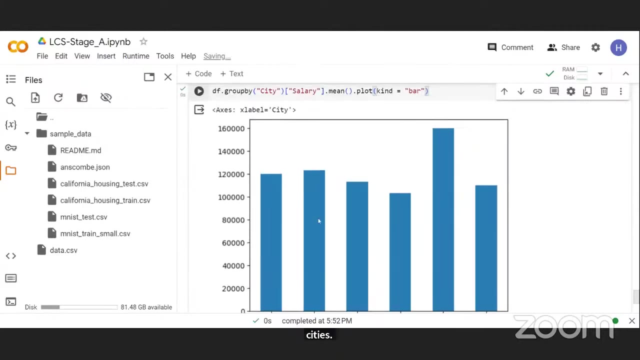 so if i do this dot plot and i say kind is equal to, i want to plot a bar chart and i want this code. you see, this has automatically generated a bar chart where i'm seeing the mean value of each of the cities. so the mean and salary for people in boston is 120 000 that of people in chicago. 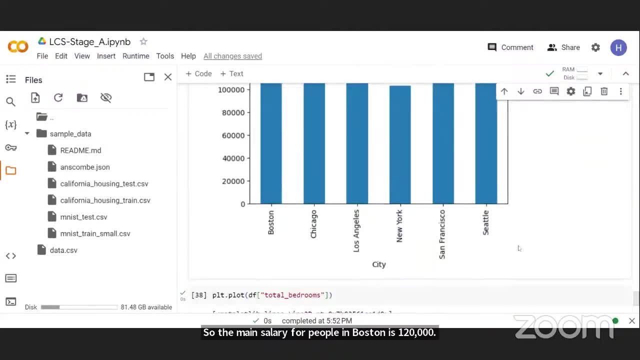 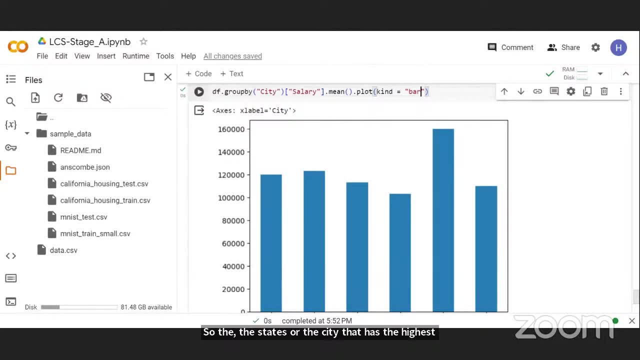 is 120 000. so the salary, the states or the city that has the highest salary is san francisco, and this is what um visualization can give us, because we just have to look at our data ones and you can make a difference. so with this now i can say that confidently, that from 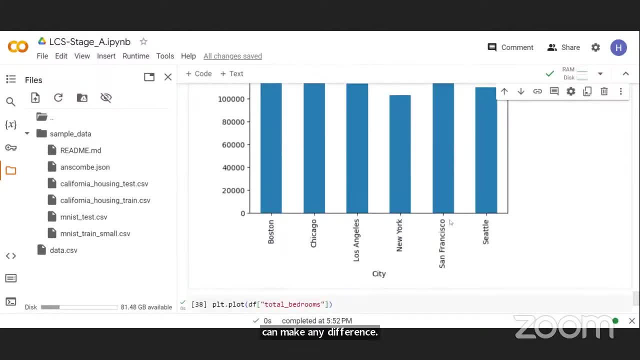 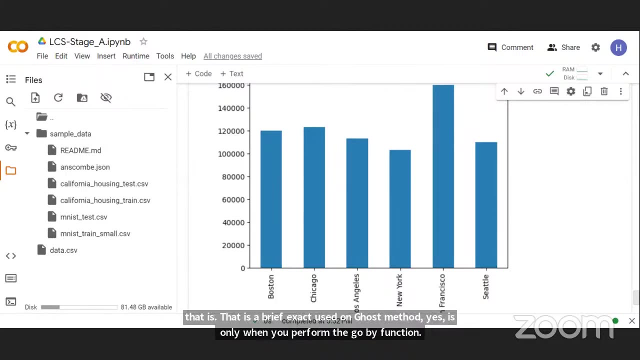 these data sets, the city that has the highest service salary is san francisco. so that is um. that is a, a brief exact used on goosebumps method. yes, it's only when you perform the goodbye function that i can start using all of these functions. another advice i give to a lot of people: 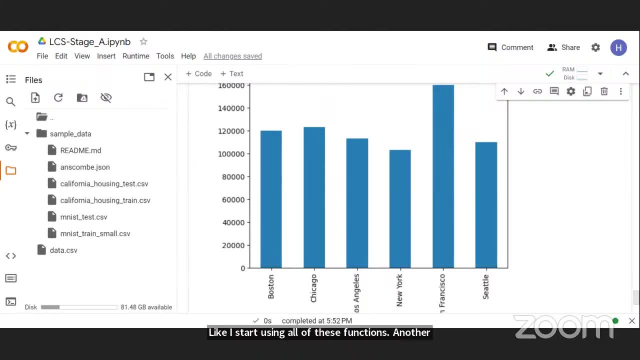 when you're starting out is you have to try and learn to read documentations, because most of these codes and libraries that we are using were not written by us. they were written by people and these guys that wrote them. they have a particular naming convention. they have a really good this. 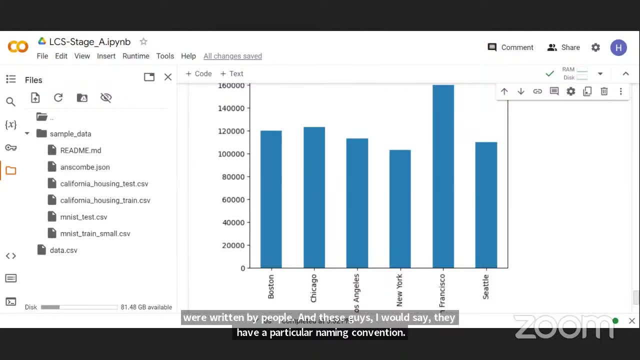 code and expect it to be used. so use them that way. that way, because then you will see actually their. so you have to be able to go through documentations of libraries for you to understand, um the functions that they wrote and for you to understand how you can begin to use these.